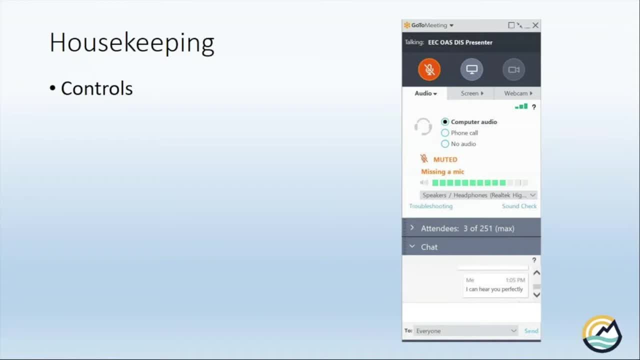 though. First thing, guys, is whether you're using the app or whether you're using it through your web browser. you'll notice there's a control panel somewhere on your screen. The first thing everybody should be aware of with it is: I have everyone muted, So you can hear. 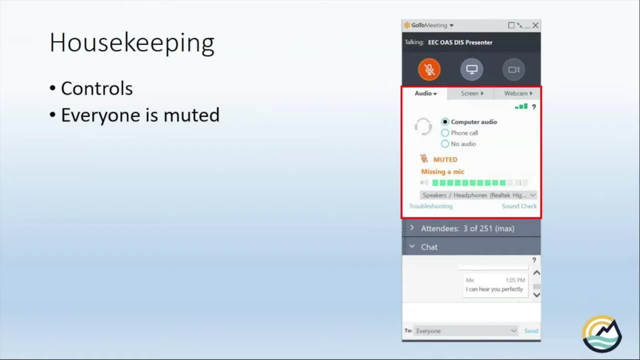 me but I cannot hear you. So if you have questions, if you have concerns, if you need something clarified, please use that chat box there in the corner. If there's anything pertinent that comes up as we go, I'm going to go ahead and have Christina answer that. 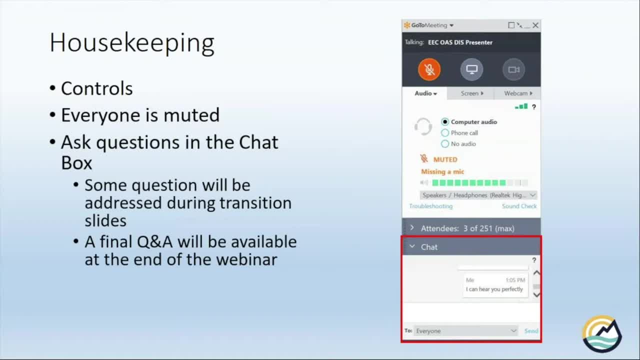 question. Okay, And then we'll do a final Q&A session there at the end. So if you have questions, use that chat box, send them in. I'm going to be moderating and collecting those and asking Christina at the end. 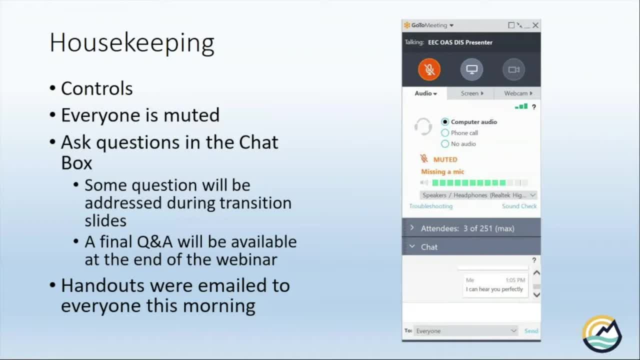 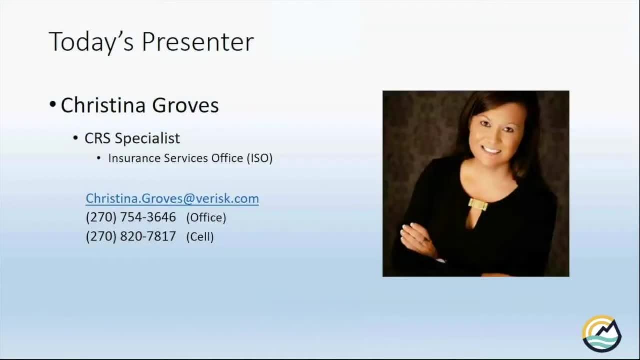 The other thing is you all, in the email this morning, had some handouts sent out to you. You may want to have those handy so you can go ahead and reference them as we go through. So, without further ado, guys, today's presenter is Christina Groves. She is Kentucky CRS. 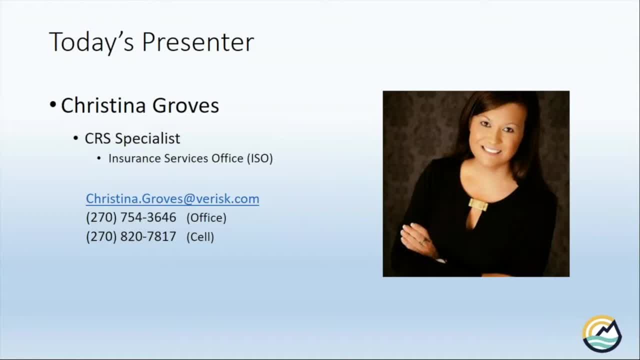 Specialist. She works for ISO, which is the Insurance Services Office. Christina has been the CRS Specialist for Kentucky as long as I've been here, so four plus years. And with that, Christina, are you still on the line? Alex, yes, I am still here. Sorry, I was muting myself. Yes, 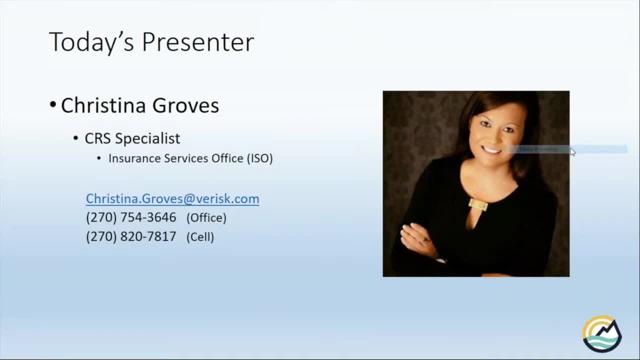 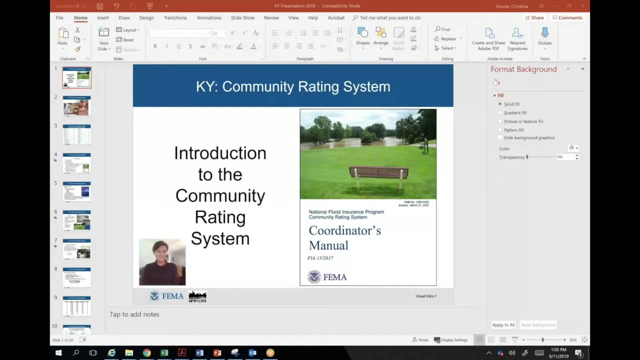 Yeah, Yeah, I figured. Okay, I'm going to go ahead and make you the presenter, So whenever you're ready, take it away. All right, So let me go to my here. There we go, Okay, Here, Does that look right to you? 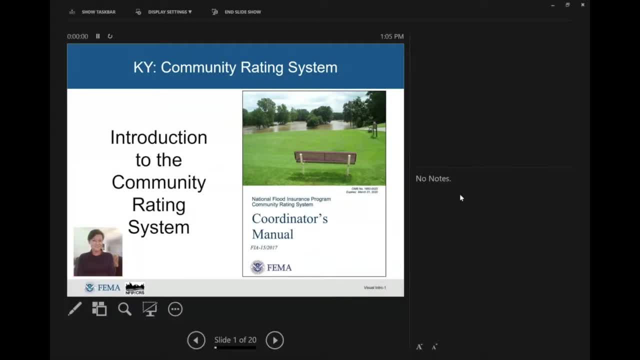 guys on your screens. Are you seeing it as like a PowerPoint would look? We're actually seeing the display side of it, So we're seeing your current slide and your next slide. Okay, Okay, so I'm not sure how to get rid. 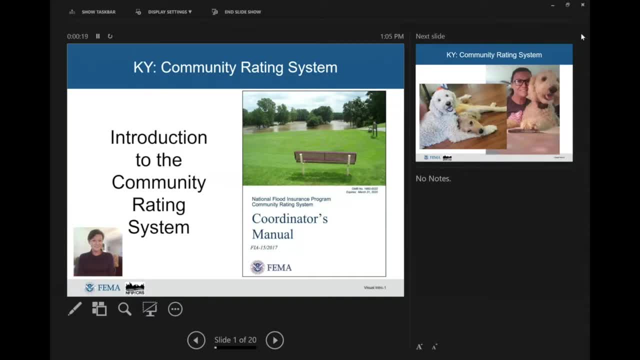 of the next slide portion. Alex, do you have any tips there? Function F8, I believe. Okay, great, Hmm, it's bringing me back. I'm sorry, bear with me one second, guys. I was going down to let me grab it here, sorry. 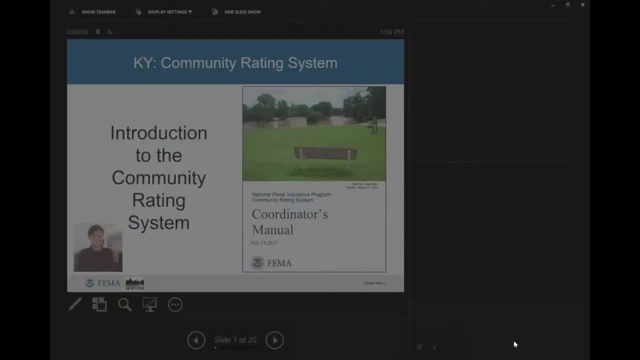 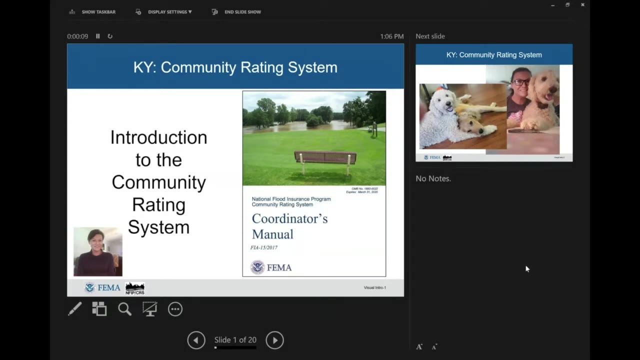 The start slide show. All right, if you guys can just live with that, I'll leave it because I don't want to waste the time trying to. I'm sorry. normally it goes straight to one slide when it displays it. Function F8 didn't. 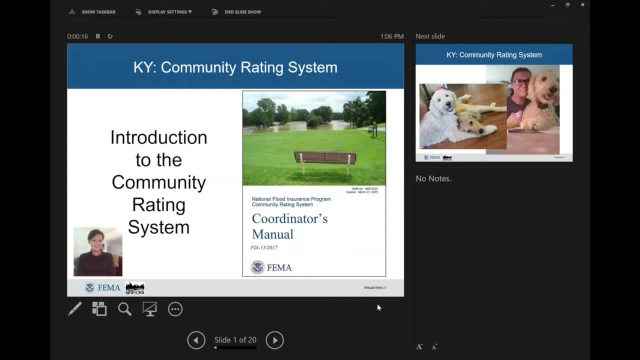 It didn't seem to do that for me, sorry. So today is Introduction to the Community Rating System, as Alex described, and I'm glad that you guys could join us. The CRS program has grown by leaps and bounds since I've been the specialist for the state of Kentucky. 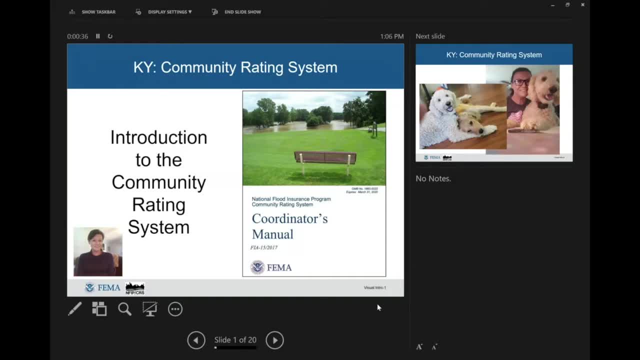 That's my gosh, and it's been 10 years now, and before that I served 10 years in local government as a planning director and a floodplain coordinator for Madisonville, Hopkins County and all the you know small communities within. 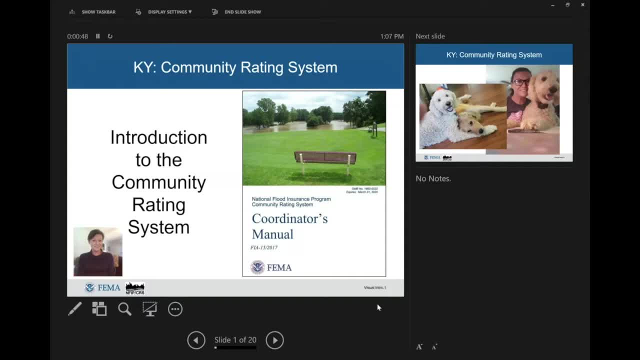 so I can relate to what a lot of you guys do on a daily basis. So what you're seeing now on the front is our CRS manual. that's currently out there. that's been extended to 2020.. We were looking at having a new manual in 2020,. 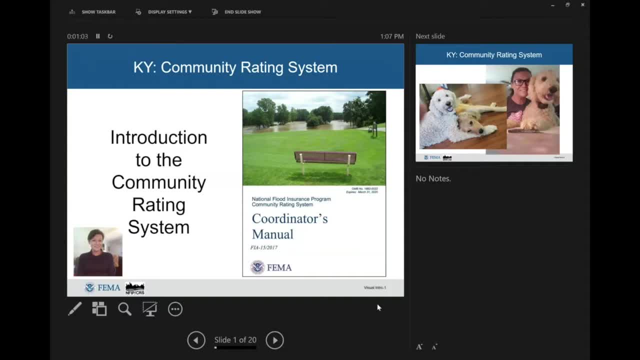 but we are pushing it out again. So you look for the CRS Coordinator's Manual when you download it. That's what the cover looks like and I'll show you the place in today's presentation to download it. A little bit of how it works for those. 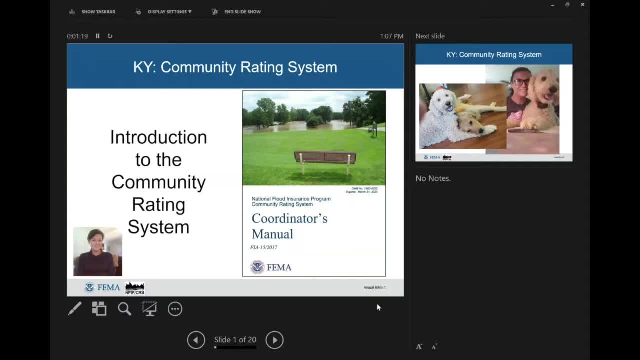 that haven't worked with us yet. We work from home and we travel to your communities. So I live in Western Kentucky, in Milneburg County, and so I'm pretty familiar with most of you guys from the CAM Conference And 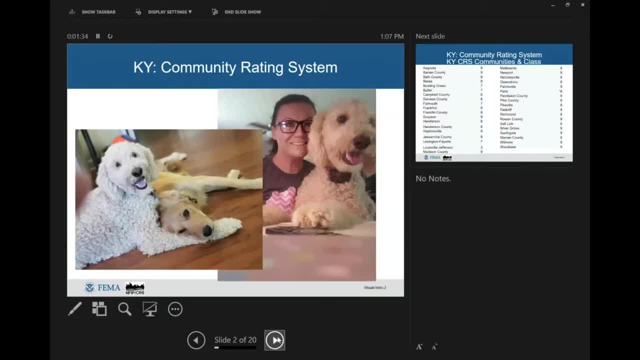 so let me go to my next slide. So this is what it looks like at my office. by the way, This is like right now. on the other end, my dogs are running the show right. So get your community work. 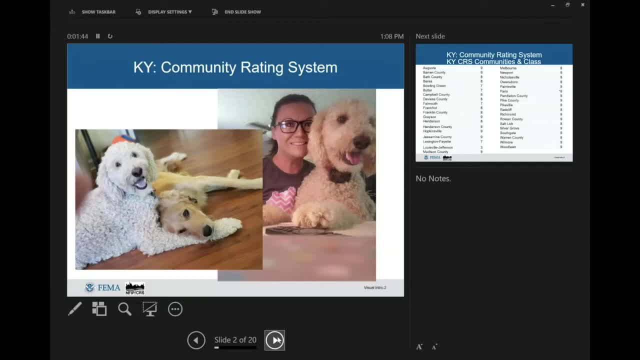 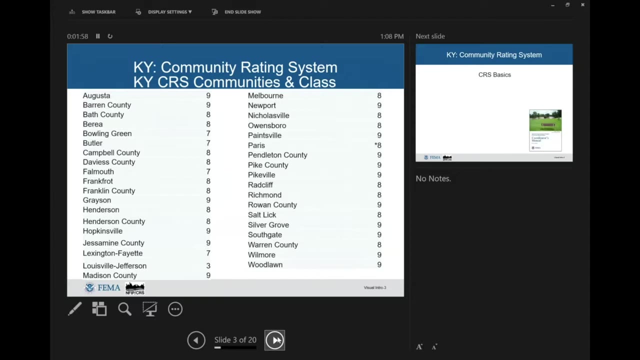 This is everyone loves a good dog. So these are my office staff. They compete every month for employee of the month is what we say for community grading. So we start to look at who's in the program, in the CRS program in Kentucky. 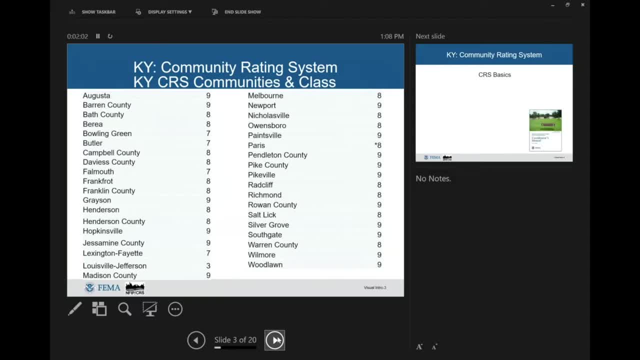 10 years ago, when I first started as a specialist, before we started to see all the overhaulings and rate increases that we are seeing today in the NFIP, we only had just a handful of a community, literally like 10, 11.. 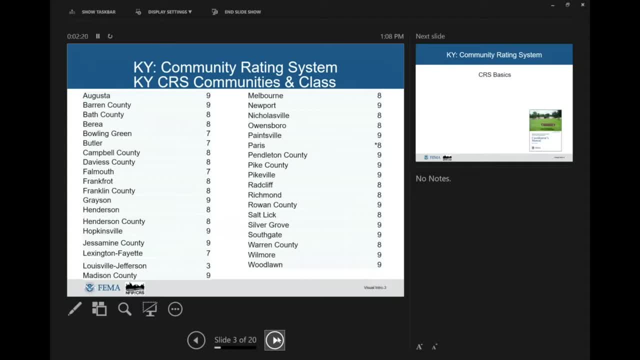 And now we're at 37,, I believe is our magic number right now And I'm super proud of the staff at the state and all the efforts on a lot of those 37 have come in the last four years since Alex has been with us. 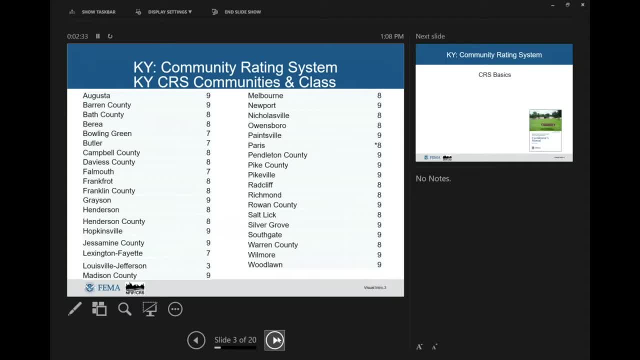 but previous to that, Kerry and the efforts that you know he continuously made to encourage the program, The more we've seen the rate increases, the growth of interest has occurred, Which is natural, And we wanna continue to help those communities to drive down the rates. 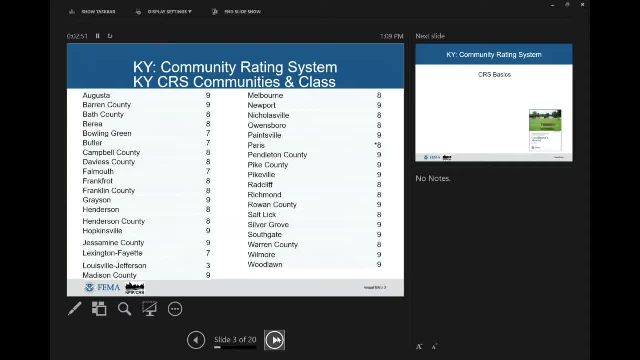 We're gonna talk about what it is, but if you're new to the program and you're on the call and you're wondering if there is anybody that's near you that maybe you could talk to, Because that's one of the best and most prevalent ways that we find 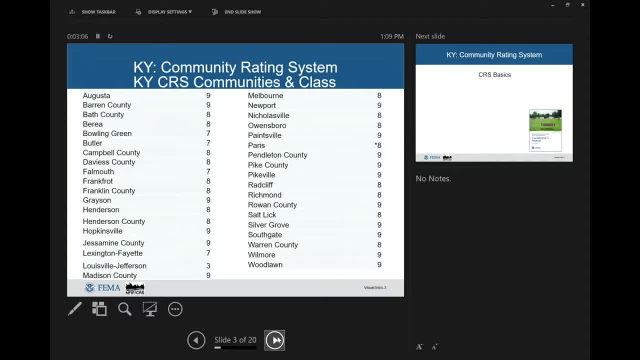 that people get information. here's a list of communities in the program Currently and their current classification, And you can see the asterisk by parent: paris. i don't want anybody to ask, um, but it's because paris is going to be moving up a class. 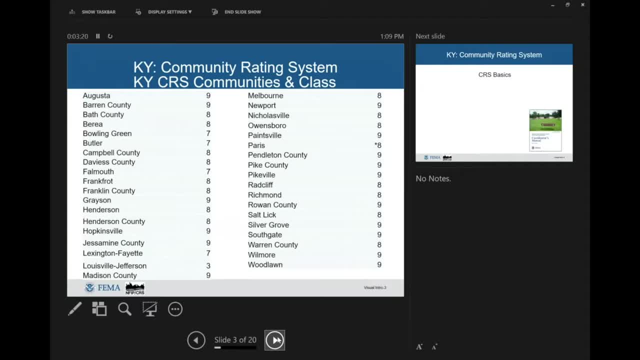 on october 1st, which we're super excited about. um, we've seen a trend of a couple class increases in kentucky the last couple years, so we're seeing people um want to see uh, lower rates by taking the next step in improving their class. so, um, take a look at the list and see if you can find a neighbor. 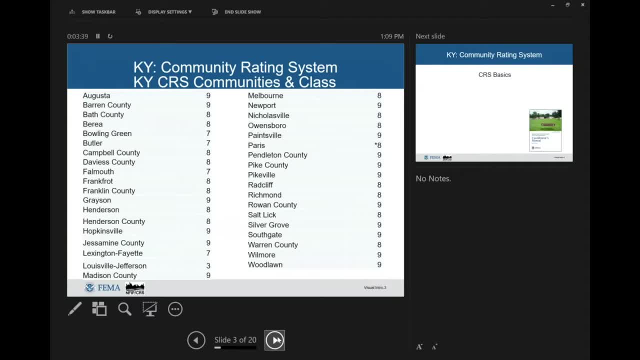 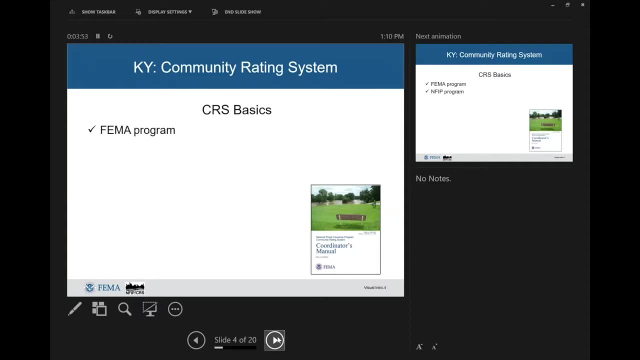 to talk to. i know that all of our coordinators have been incredibly gracious to say: please tell people to call me. i'm glad to talk to them about it. so, uh, always visit that. um, the basics of crs are that we are a fema program and we are under the umbrella of the nfip. 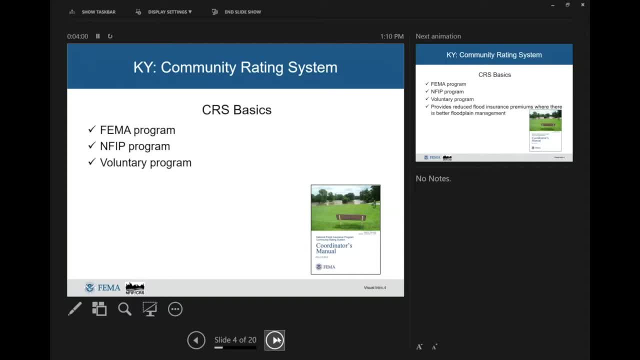 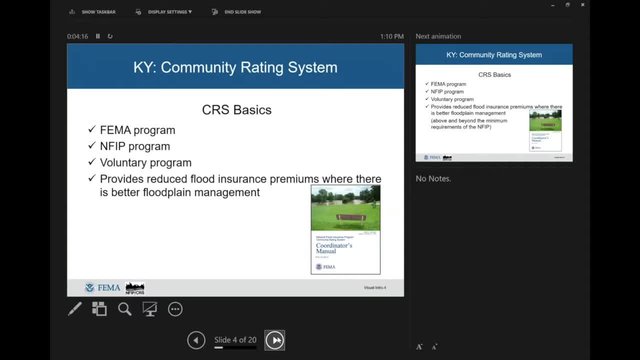 through your efforts of higher standards and better floodplain management in your local jurisdiction. the uh- basically you're being rewarded for the above and beyond and going doesn't be on the minimum of the nfp. so i think of that as the minimum nfp would be. 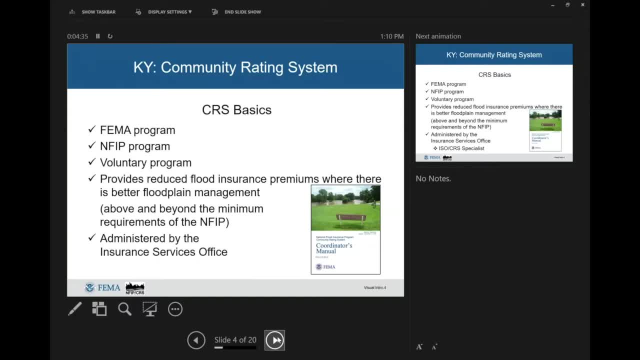 the build to the base flood elevation. but when you adopt freeboard, you're practicing a higher standard and we're rewarding you for that by recognizing that you're adding that extra element of safety and public protection and then also minimizing risk at the same time. so the crs program is administered by the insurance services office, iso and most 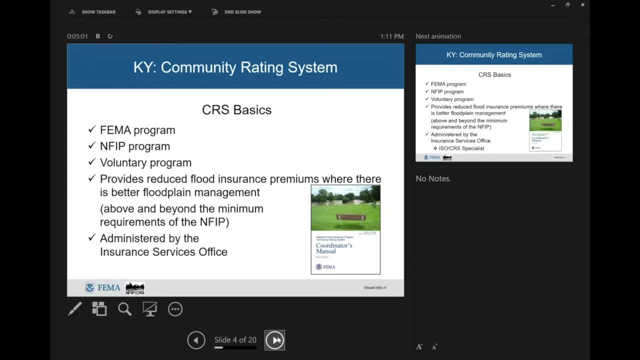 people are familiar with iso via the fire department ratings and that's something that's one of the oldest rating programs in the country. um, and the federal government models the rating system and the administration of the crs rating after the fire program in its effectiveness. the field specialists such as myself are known as iso crs specialists that we visit the communities. 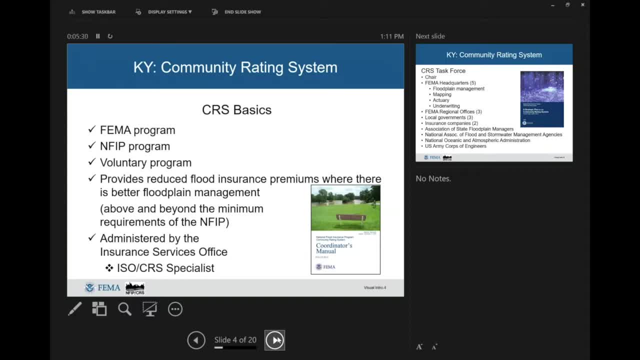 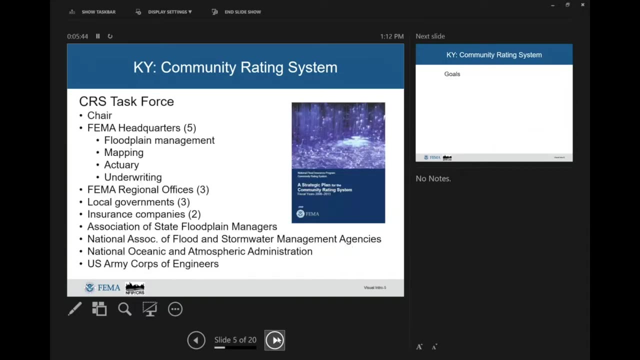 work with you, help you administer your program and realize the discounts in your community. those are just those basic points for crs and we go on to how is crs monitored? where do these rules come from? so we look at the crs program has oversight by task force and the task force is made up of the group that you see listed on your screen. 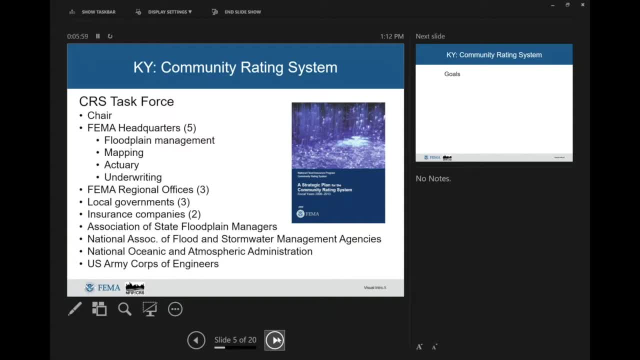 that group um very diverse but also very much speaks to the heart of all these entities that are impacted and have feedback and also have benefits, like the us army corps program and the fire department. they're a good example of a group that's not only for малcon's fhs but also not for 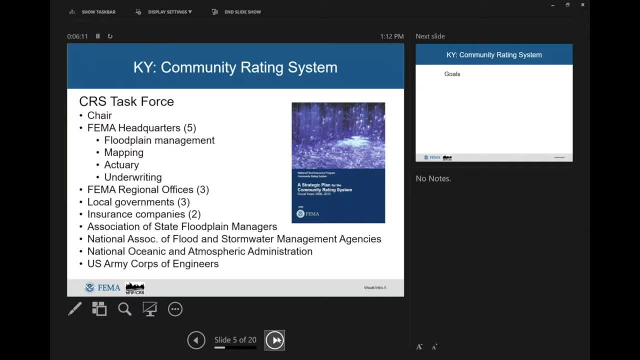 all of the other communities in the area of fire departments because they do not have a group that is going to assist the community if they are being purple. wishes to use firemen as a resource are of local management. they don't need to be on fire, they need to be in the area of fire. 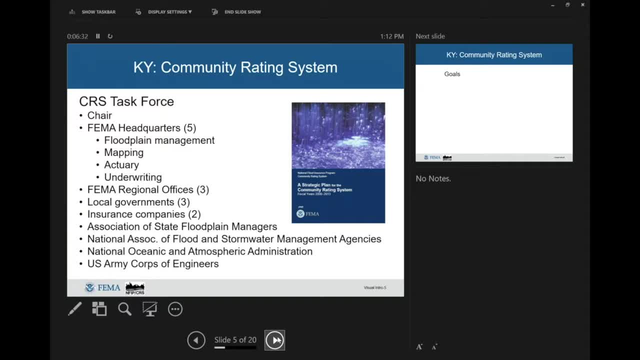 or fire incidents or fire systems. they need to go to a place that is in the area of fire and so they can be in the area of fire. but they don't have to have a group of firemen, and so they can do. they need to go to a place that is in the area of fire and so they can be there with their 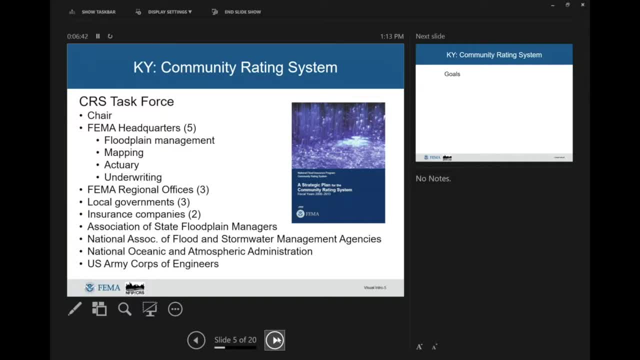 family, and so that's the part where they do the work they do in that area and so you can see they're can see on the list. We always encourage folks that are interested in the task force to reach out to us so that we can always provide your name if a rotation ever comes open and they start. 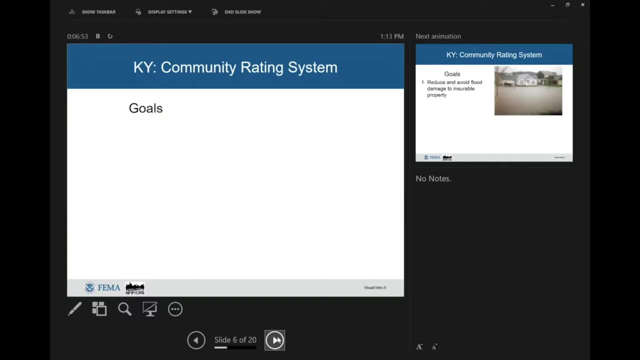 looking for candidates. The goals of the CRS are three goals and they mirror the goals of the National Flood Insurance Program. The first goal, the most important, maybe to reduce and avoid damage to the insurable property. That's the first and foremost, because that helps to stop. 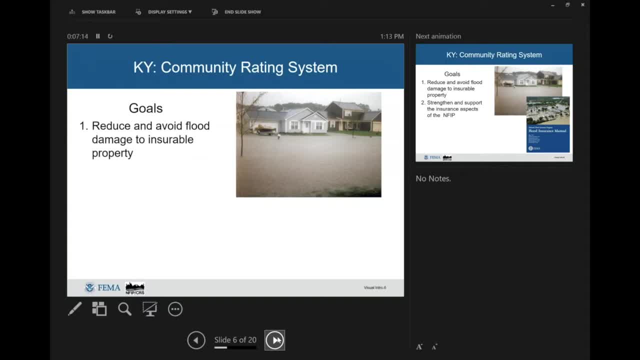 the interruption of life and helps to lessen the burden on folks that receive those losses. So if you can get someone to raise their finished floor by applying a free board regulation throughout your community, perhaps when that 100-year event comes from their floor would not realize that. 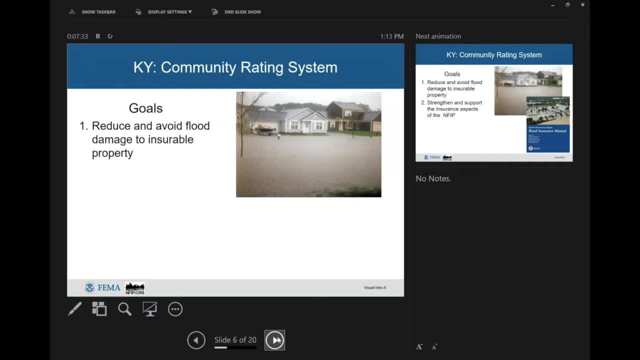 inundation and therefore there would be no damage. we hope There would be. you know, also no claim to the National Flood Insurance Program, but also for those who do not have insurance also still have that protection. So first and foremost, reduce and avoid damage to. 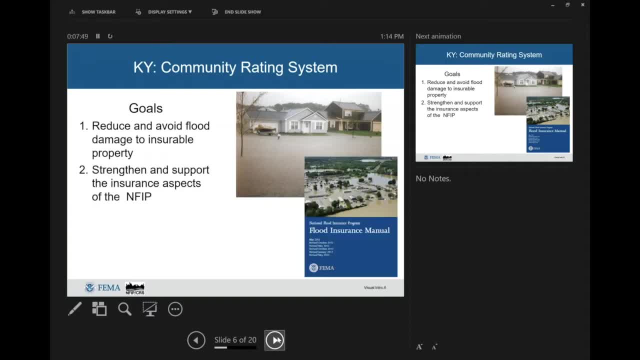 insurable properties. The second goal is to strengthen and support the insurance aspects of the NSIP By lowering the rates. we hope that encourages people to purchase flood insurance to make it more affordable and more affordable. So that's the first goal. The second goal is to 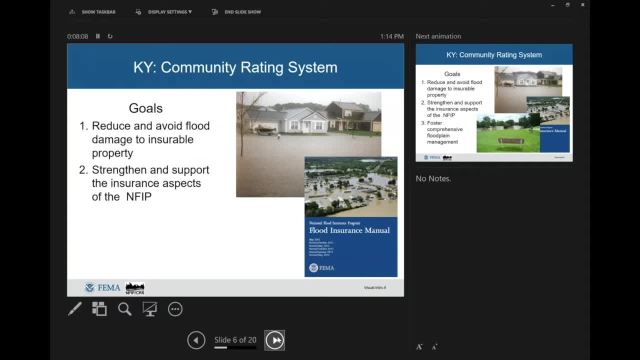 We hope that you know, as a community, that you, making those efforts will then promote the purchase of insurance for the constituents in your community so that they're able to protect themselves, because that first and best level of protection for anyone is that flood insurance policy. 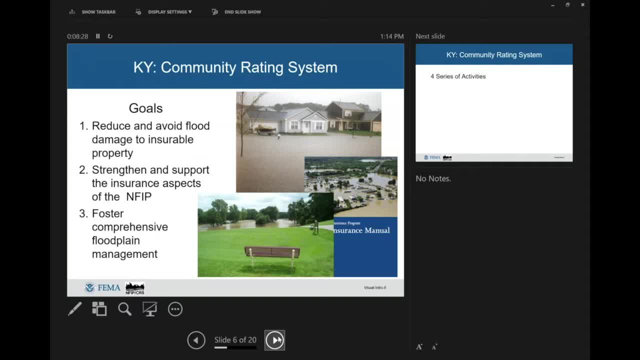 Lastly, it speaks to fostering a comprehensive floodplain management program, Community upon community that I work with and speak to after the fact in conferences and in follow-ups, they say that being a part of the CRS makes them stronger, it makes them better, it makes them practice. this documentation, which can be minimal but it does not go without being said: We are a documentation program and it does fall in the community to document it, but that practice makes you really put into place. 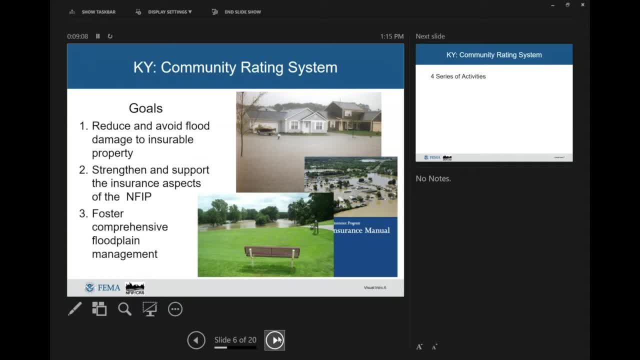 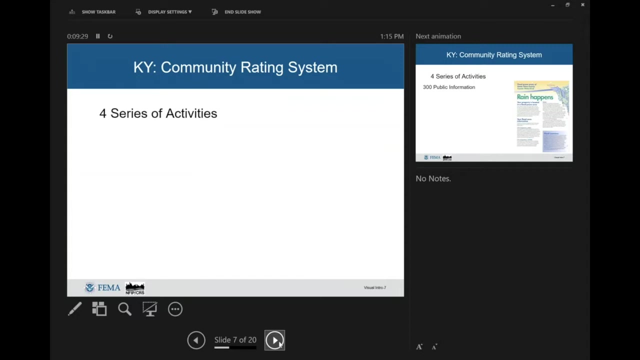 a comprehensive program. It makes your program stronger. And then communities then say it springboards them to want to do better and to increase. and as people start to realize those discounts then they begin to further push for higher standards and more protection. So those are our three goals for the CRS program. We're based on four series of activities. 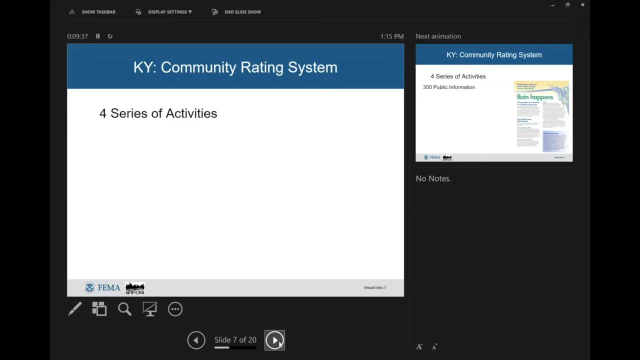 This is where I like to remind people that those four series of activities are in that really big book, the CRS manual. several hundred pages. It's big, it's heavy and it's intimidating, But the best approach that I recommend for anyone new. maybe your community is not in, so you're new and you're thinking about joining. 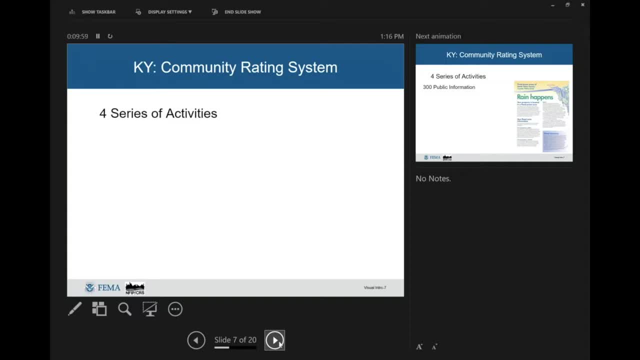 Maybe you're a new floodplain manager, a new coordinator, and you've inherited a community that's already in the program, So it's new to you. There's lots of folks that we come in contact with that say: hey, I'm now the floodplain manager for Community X and I've never worked CRS before, and this manual is a lot. 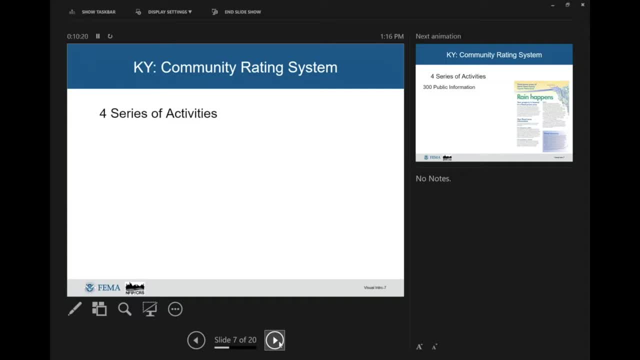 So we remind people, use the manual as a reference. Use it as it's broken down in a very streamlined way, which we'll talk about, But use it from the point of view that get to know the activities you're getting credit for. 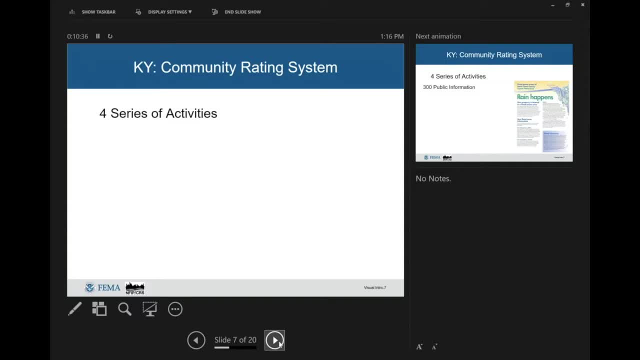 Get to know. Read the slides. Get to know the sections you're getting credit for. Read the sections that you might want to apply for credit for. Think of it like this: You may never, ever be a tsunami-ready community here in Kentucky. 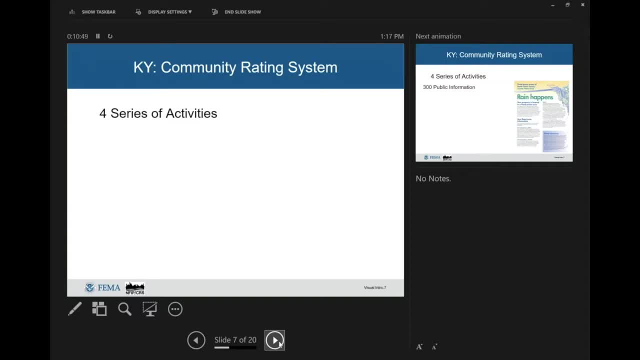 So, therefore, why should you maybe spend the time studying that activity per se when perhaps you have a levy in your community and you might want to visit that section in the manual to see if it's credit-worthy for you? Sorry, the wrong button. 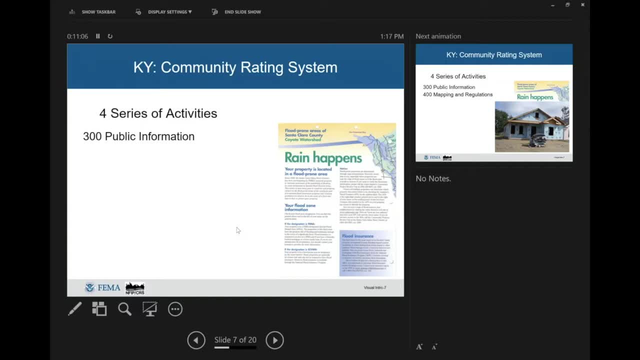 So the four series of activities. The four series of activities are numbered and it's the 300 series, the 400 series, et cetera. The 300 series is public information. So the heart of that would be your elevation certificate. 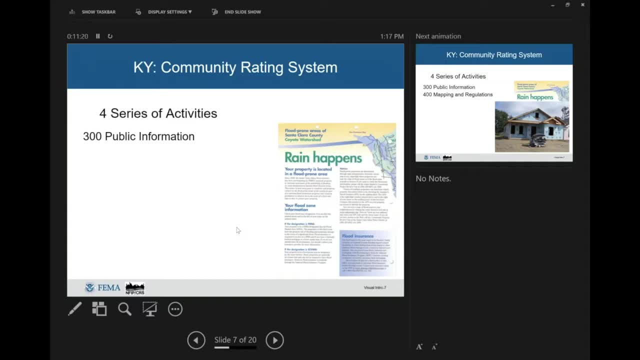 You think about your outreach project that you might elect to do. Think about something as simple as- and I can point to this in Kentucky as a former planner myself- that, on your plats, many communities in Kentucky require on a minor or a major. 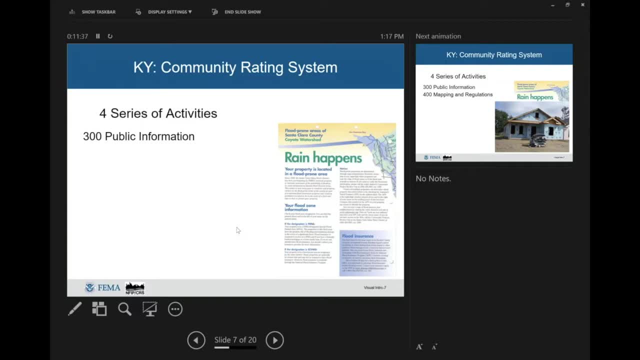 Plot for land divisions, to have a note that says if that particular parcel being impacted is in or out of the floodplain on that current effective set of maps. Perhaps they even go as far as having the surveyor or engineer show the boundary on the map, on the plat that's being filed. 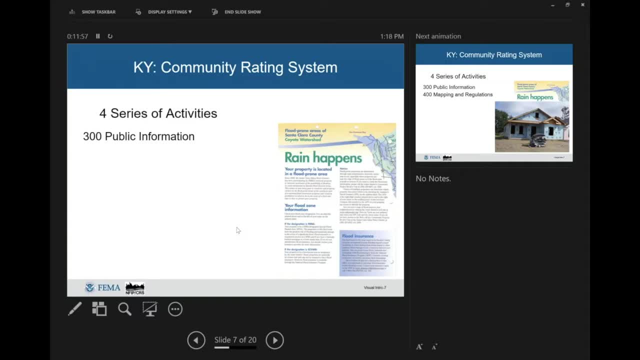 That's a piece of public information. That's also a creditable thing in our CRS manual and most communities have that as a part of their subdivision regulation. But think about it: How are you informing the public about flood hazards, about information that's available, things on a website, things in the library? 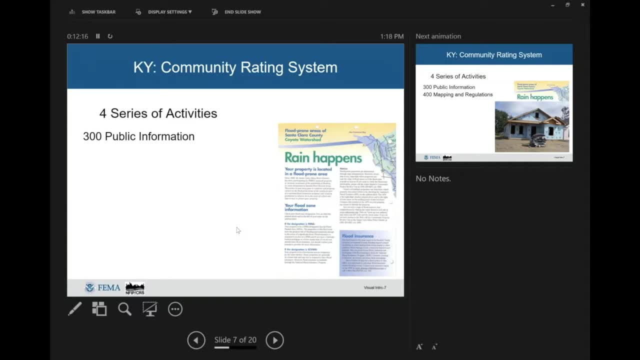 That's really what this is about. 360 is about. if you get that phone call that says my driveway tile is flooded again and having a drainage problem, could you come, And usually as a community, you one receive that phone call. 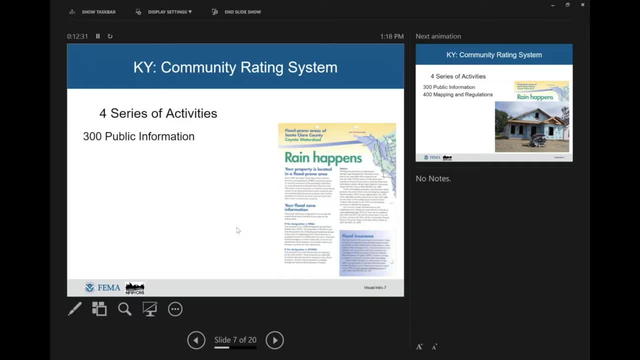 You two then oftentimes go out and make a site visit, So look at it and give them advice. Sometimes it's because the neighbor is doing something crappy and it's a civil matter. Sometimes it's because maybe there's something blocking a tile, causing backup or something, and it's something the community can do to assist. 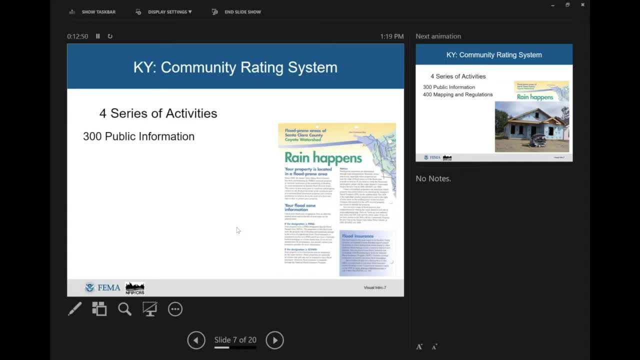 Either way, you've offered assistance to the public about a flooding issue, public information. So those are all things that, with proper documentation and meeting the criteria in the manual, could receive credit and are all things that I feel Most every Kentucky community probably does some version of, and oftentimes it's some version that they can just tweak and document properly to receive those credits to lower or work on lowering the flood insurance rate. 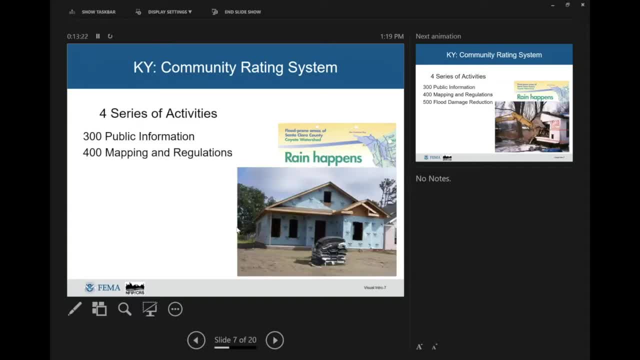 The 400 series is mapping and regulation. When I say that, I want you to think about two big things. It's your maps that you get from FEMA in the state and perhaps what information you fit into. It is also your flood ordinance. 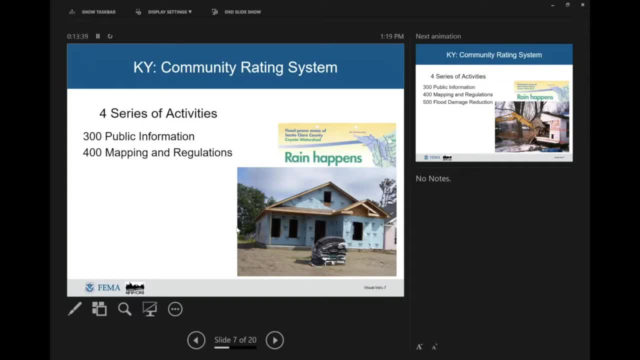 Those are the two big pieces of the pie, but it's not all of it. This, also in the 400 series, would include your GIS credits for having a working GIS system, and it doesn't have to be one you own. I know in Kentucky many cities and counties are partners and sometimes it's a regional partner. 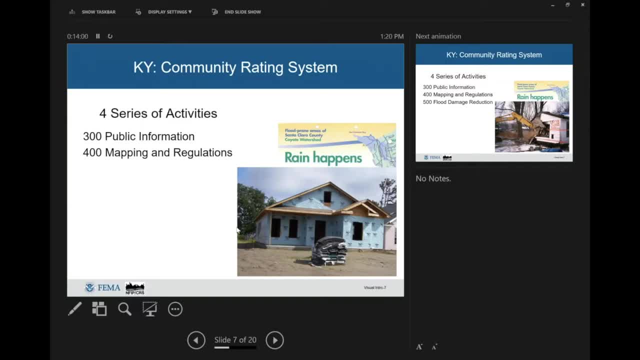 The state of Kentucky has the flood portal, the map portal, and it's wonderful. It's a tool that some of my communities that don't have GIS in-house or a partner in GIS- some of my smaller communities- actually take credit for the state flood risk map portal. 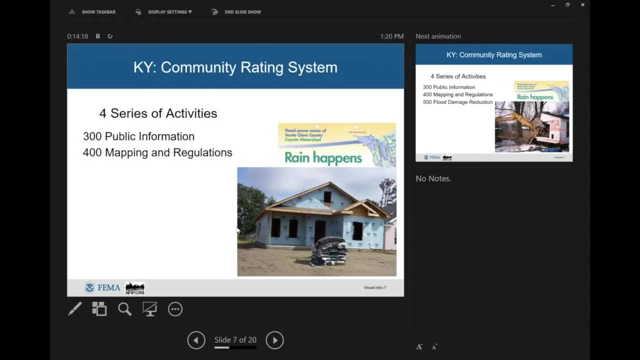 There are many avenues. you can use up to three GIS systems to obtain these 140-ish points. so they're out there. So stormwater is also under mapping and regulations in the 400 series. Open space is also under mapping and regulations. So stormwater is also under mapping and regulations in the 400 series. Open space is also under mapping and regulations. 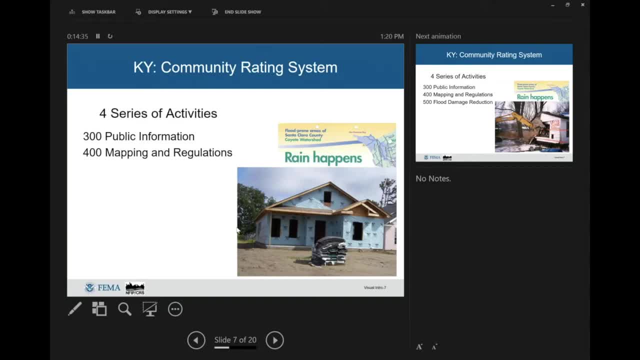 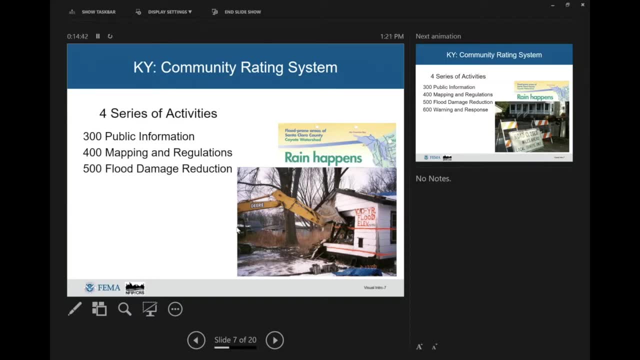 A lot of things under that broad title of the 400 series. 500 is flood damage reduction. That's where we would think about addressing our repetitive loss, And there's always that misnomer out there that we want you to mitigate all your repetitive loss, or that we require you to mitigate all your repetitive loss to be in a program participant. 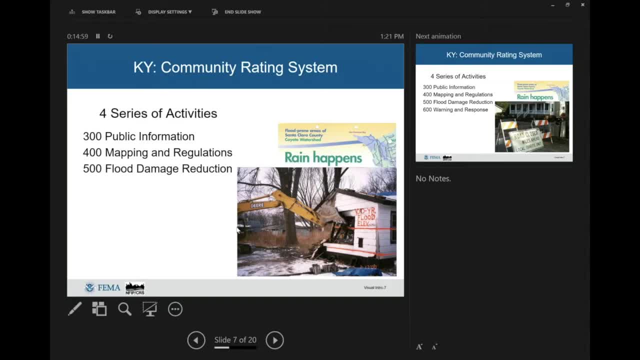 But that's not true. We do have requirements that you have to provide information to them. You have to take a look at Some general areas around them that we do not say you have to remove them or elevate them to participate. Certainly, if you remove or elevate, there may be ways that you can even realize credit for that. 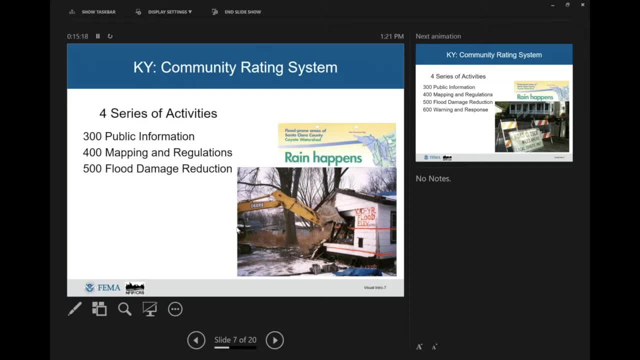 Under this same 500 series, everybody in the state would be participating in a flood. a floodplain management plan of some sort. Usually it's known as the hazard mitigation plan. They're generally regional, conducted through the area development district in most cases. 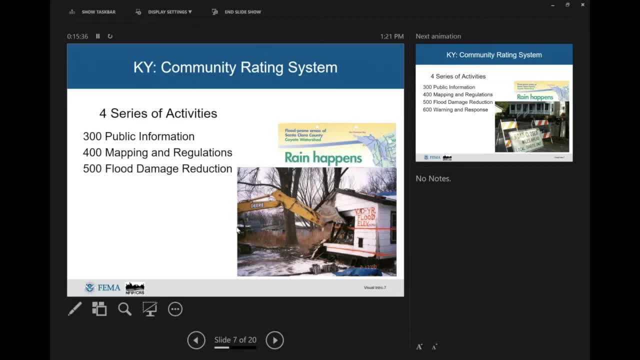 And those if meeting the requirements and a well done plan could realize anything from 100 to 200 points on average and it could be upwards of 300. But those are. those are those really highly invested, almost individualized to the jurisdictional plan, but still is credit worthy and something you're participating in. 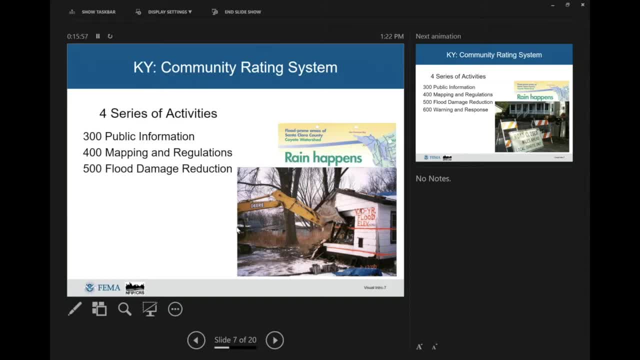 And if you participate to the criteria, it could be then transferred over on working towards reducing the flood insurance rates in your jurisdiction, And that's where we would look at that. And that's where we would look at that. And that's where we would look at that. 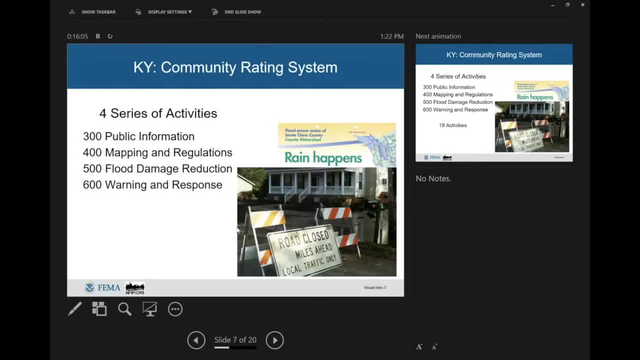 And I will say the 500 series also includes your buyout if you've been part of a buyout program, especially on the eastern part of the state where the court did some work also for elevation programs. So not just buyouts, but any time we've elevated or protected a structure you may be eligible for credit there, including drainage maintenance as well. 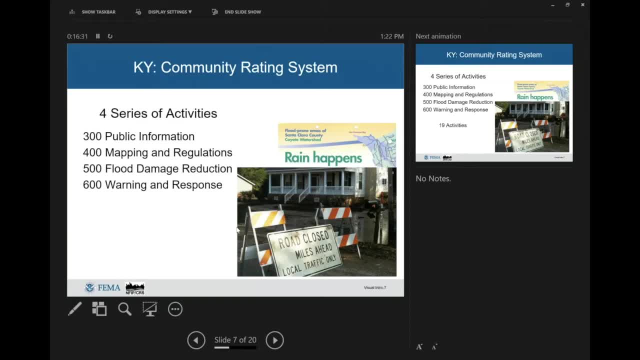 The 600 series we're looking at. We're looking at warning and response. So we think about our emergency management And so often, oftentimes, we go to a community and we don't get a lot of people to buy into the emergency management credit. 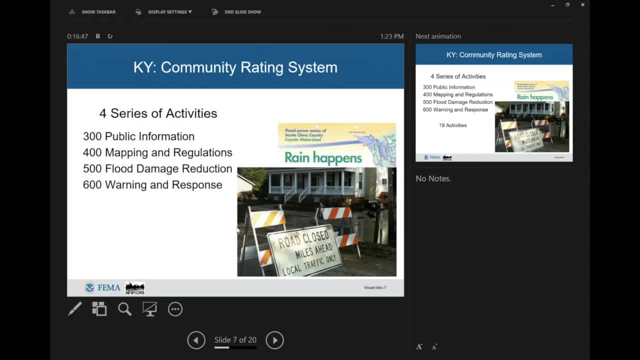 That's related to that And it's manual, because Emergency Managers think this is flood insurance. it's not for me And it's not what we do, But we give a lot of credit for what your emergency manager does on behalf of your jurisdiction. 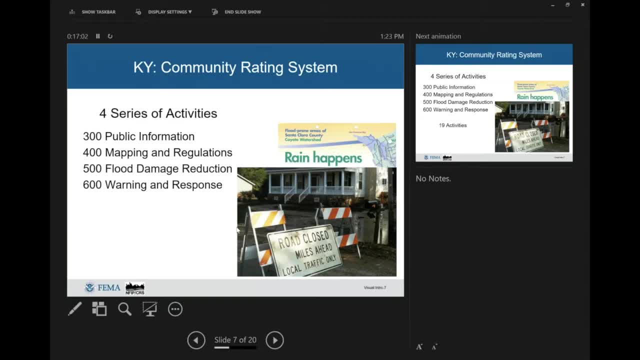 So it is absolutely that we dedicate a whole. So it is absolutely that we dedicate a whole. So it is absolutely that we dedicate a whole activity to the emergency manager and their warning and response and dissemination and all of the activities related to what they do to warn and then, after the fact. So please, if you know, 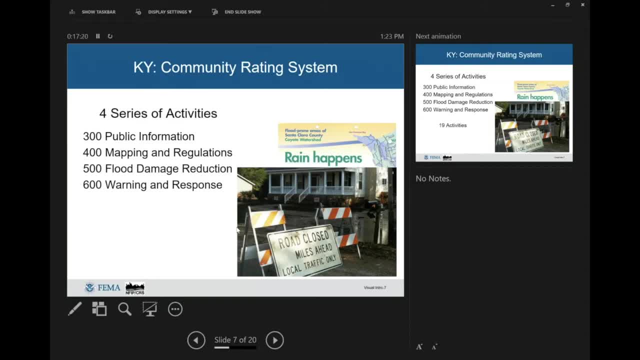 you decide to apply, ever involve your emergency manager. I always tell people, invite them to the meetings, get them talking to us, because I think they'll find that we very much are interested in what they do. and it's not just about flood insurance, because this program looks at your 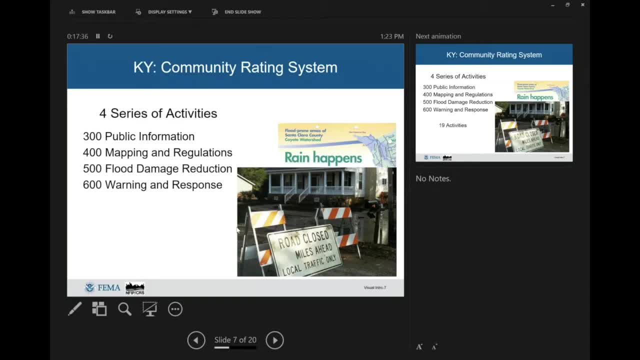 community as a whole, not just the flood portion. This activity would also include credits for levees and for dams and there are some communities that are eligible for credit on behalf of what the state does for the state dam safety program. If you're in the inundation area of a 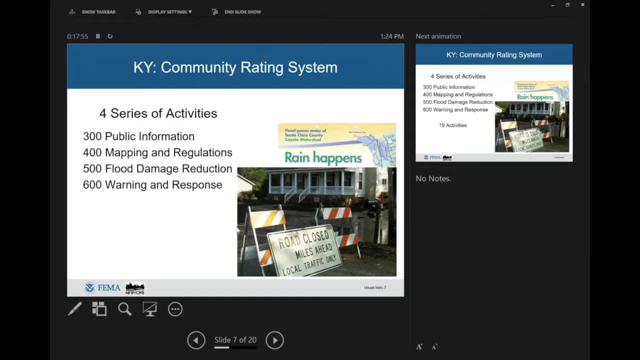 potential high hazard dam and that doesn't even have to be in our state you could. Wolf Creek Dam is. if in a breach, then Nashville would be in the inundation area, so they can take credit for Wolf Creek, even though we're, you know, four hours away in that scenario, but it would impact. 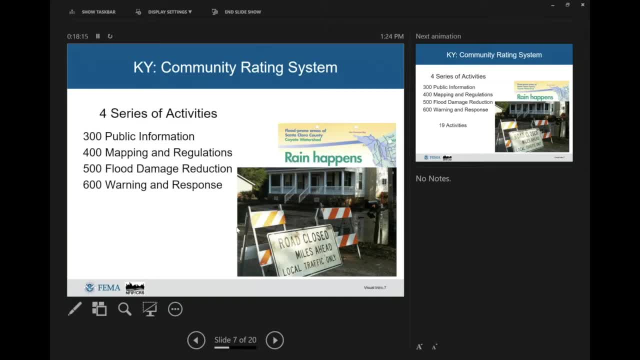 downtown Nashville. So, for example, that is one of those cases that we want to have those conversations and learn about your community so we can try to find those places to award credit. In those four series of activities- the 300 through the 600, that's broken down into 19 activities which I kind of give a brief. 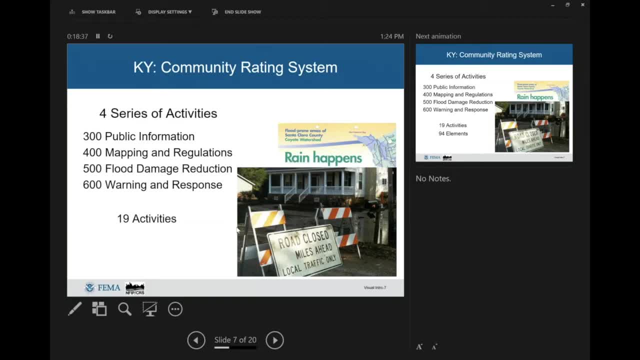 summary and the high points on. so if you imagine it goes, 300, it's the public information. 310 becomes elevation certificates, 320 becomes map information service, 330 becomes outreach. Each one of those series has that following layout of breaking them down by tens and by: 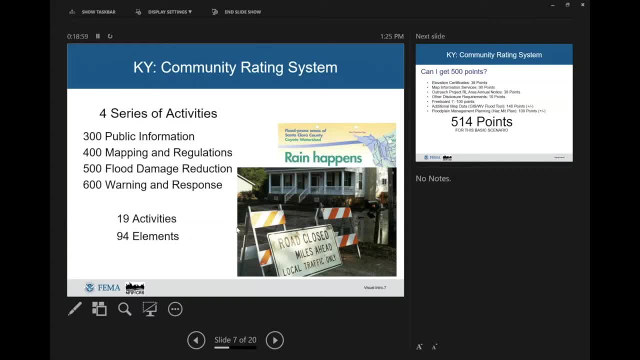 activity. Again, there are 94 elements that go under those 19 activities and many, many sub-elements that go under those. What I really want you to hear when I say all that, though, is the important message is: my job is to know the manual. 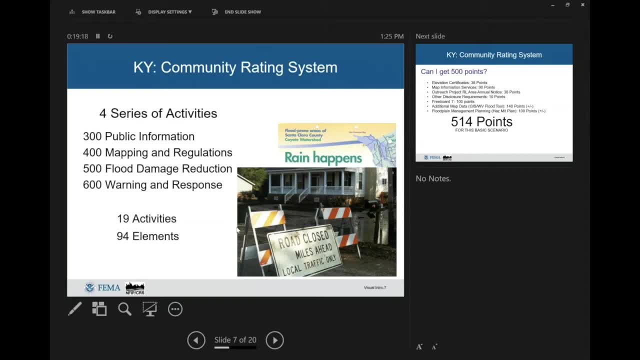 My job is to help you guys get through this. My job is to be a guide, and Alex is as well, and Alex is really well versed in the manual, so you have a lot of resources that you don't have to go through. 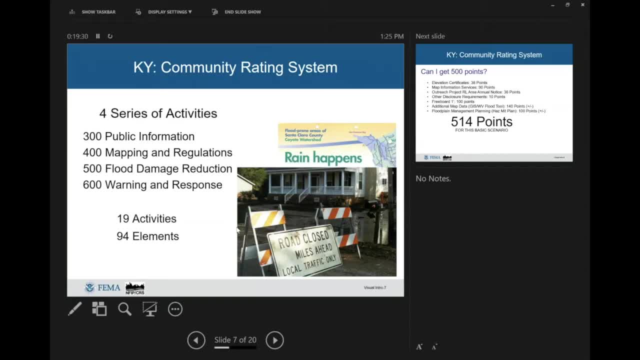 I have to take that 600, 700 page manual and commit it to memory that you can begin to, like I said, familiarize yourself with it and then follow that manual as a guide and say, Christina, I'm thinking we might be eligible for credit. and let me talk to you about the nuances. 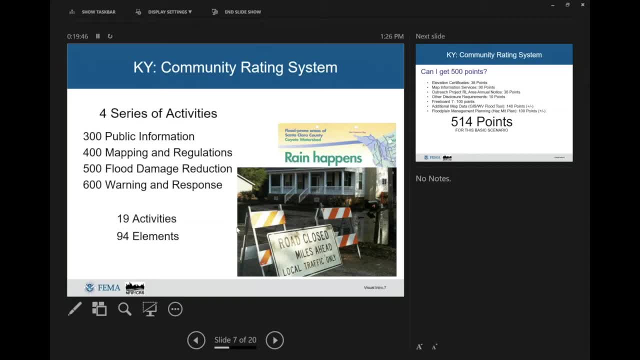 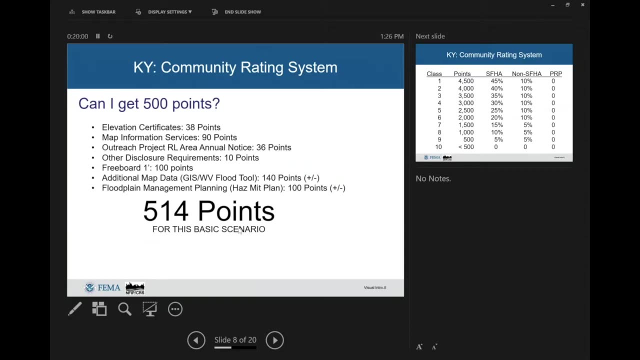 in the manual so that way you can still try to maintain the other 28 jobs that you have in your local government, because that's often. you'll wear many, many hats and we realize that I'm deciding today. we were going to talk about an introduction. I wanted to talk about if 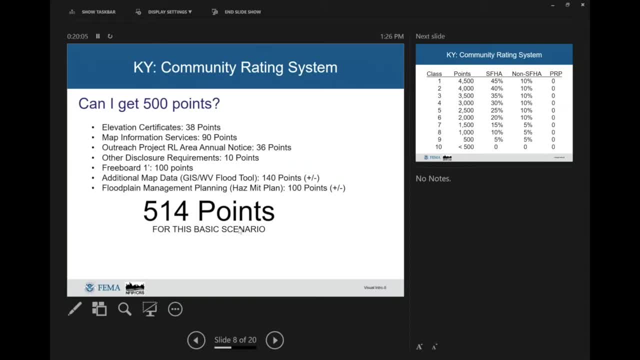 you're in Kentucky, could you get that first 500 points- and I'm going to show you in the next slide that there's a scale to this and that we're aiming for 500 points. so actually I'll flip over and show you and I'll come back. so this: 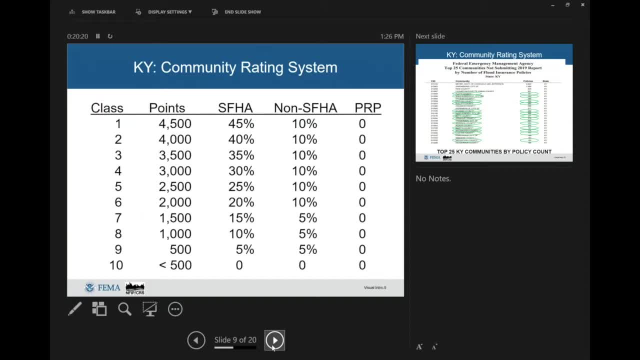 is the scale of classes. it starts at a class 10, everyone's a class 10 until you get into the program, and class 10 is no discount, going to a class one being the 45% discount on a floodplain policy, and you can see all the classes in between. 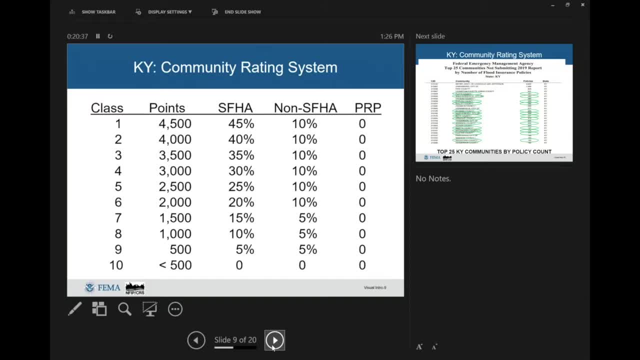 it's a 500 point increment for a 5% discount. you can see that the SFHA would be for your policies, for those in the actual 100 year. the non SFHA would be those perhaps a 500 year or not in the flood, not mapped in the floodplain. 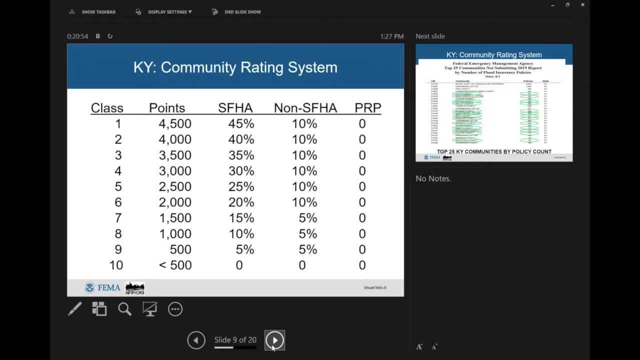 there in the second year, so we'll be looking at that in a little bit more. zonex, the prp, is the preferred risk policy. um, right now you know they're getting the best rate there is. there's currently not a discount on those policies, though that is being discussed. 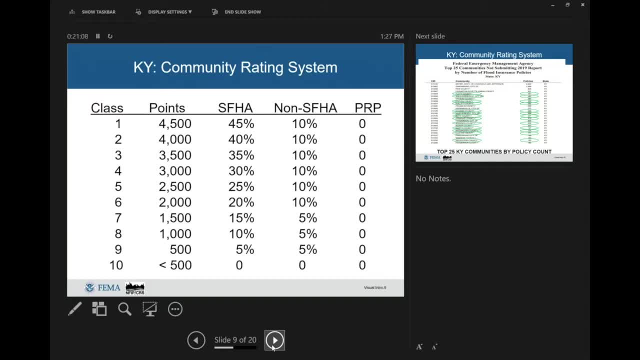 at various levels. um, they're they're looking at putting a discount on the prp or on contents or something more to encourage those outside the sfha to go ahead and purchase policies as well. so that could be as something we see the needle move on in the next few years, possibly, and it would be. 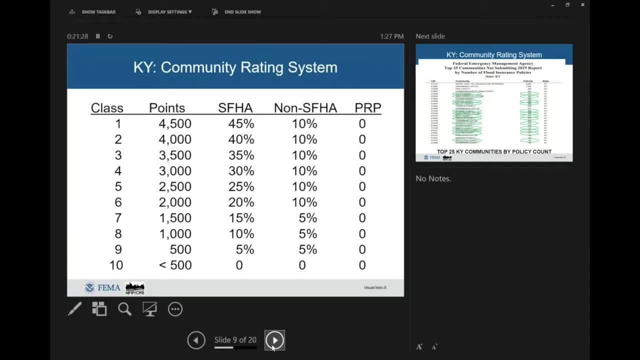 further encouragement. it'd be wonderful to see a discount come on a prp if that happens and the prps are the ones that you're going to really see in that commercial. when you see a commercial on tv that says you know, you can get flood insurance for as little as maybe they might say 350 a year. um. 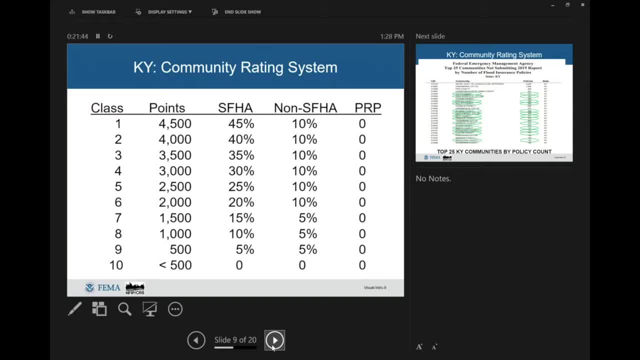 that they're referring to a prp policy in most cases. so we're trying to achieve 500 points and we want to work our way up in 500 point increments to get to different classes. so if you remember, our slide is a list of kentucky communities we were able to see, like louisville as a class three. who's? 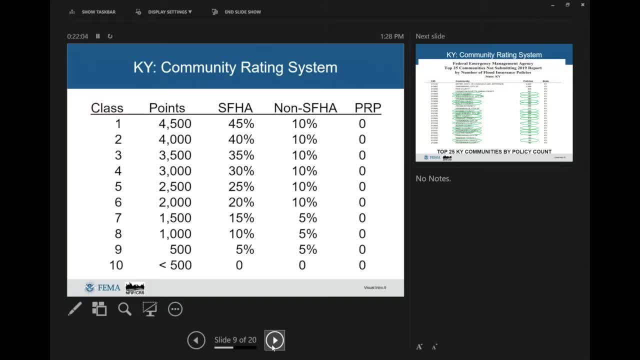 you know taken 20 years to work there, and diligent and and great work. and we see um, like bath county and salt lick, who started as a nine and one in one year went to an eight, so went from like five percent to ten percent. uh, richmond was one that recently went up in. 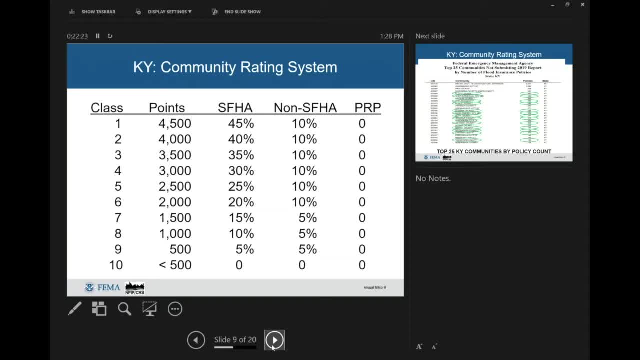 kentucky and um, they were able to get a discount and and they got their foot in the door and they got their basic credit. and they got their basic credit and then they had, um, increased their higher standards, they increased their free board, i believe is what memory tells me- and, uh, we're able. 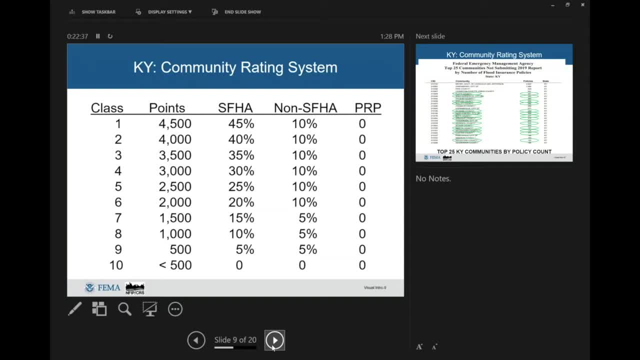 to realize a percentage, a discount increase for their policy holders. and so there have been others, paris like that's where they're moving to that eight on october 1st. um, so 500 points in kentucky to me. i'm sorry i went the wrong direction. 500 points in kentucky to me can look like 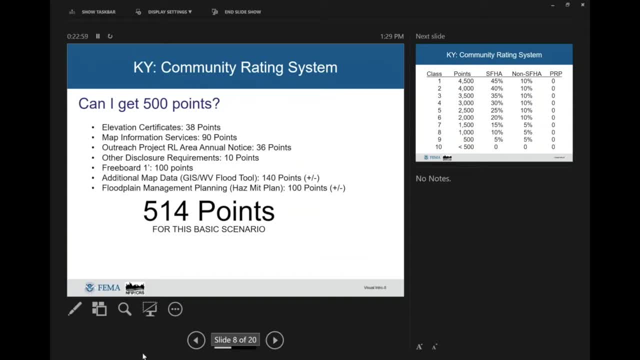 this. um, i should have put activity numbers out beside those, but 310 is elevation certificates. by joining you're going to get that 38 points the first time by agreeing to collect finished construction elevation certificates on new construction and substantial improvement in the 100-year floodplain, the 100-year sfha. so you're going to be verifying it anyway. you need. 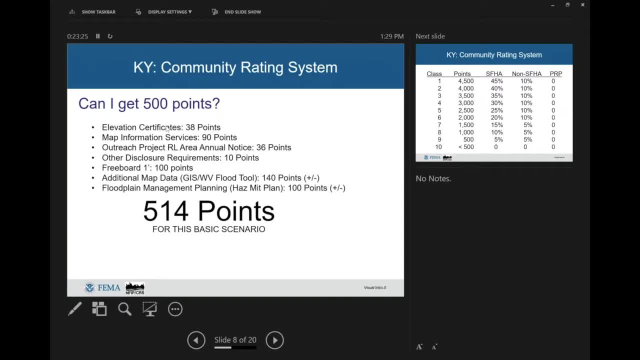 to verify where your finished floor is on new construction, substantial improvement, really more and less any construction that we're looking in this program at the new and substantial um. you're going to collect that verification, so we want you to collect it in the form of the current. 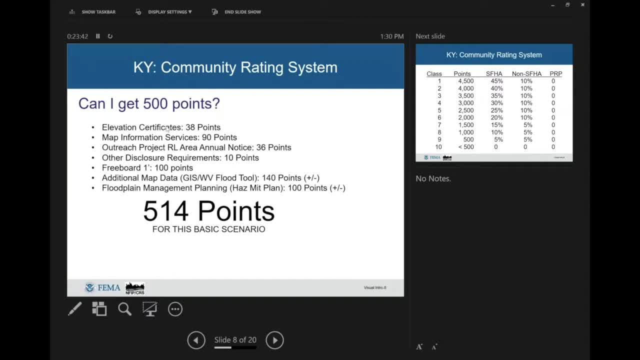 fema elevation certificate or flood-proofing certificate, if that is the applicable type of structure and activity that's happening? um map information service is 320 worth 90 points, and that's for when people call you contact you. am i in or out of the floodplain? um, can you tell me a bfe? if it's? 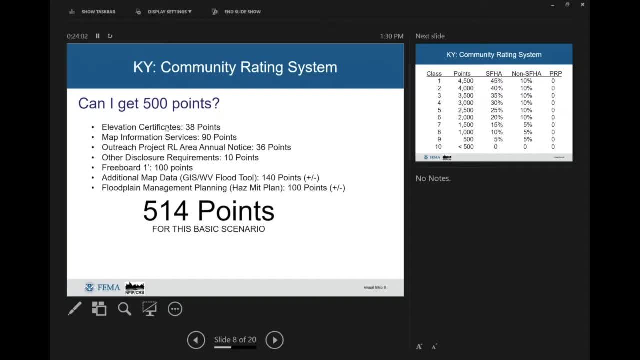 available? can you tell me if there are any wetlands on that site? can you tell me if it gets to the 100-year flood, about how deep is that going to be at my house, and can you tell them that information? it's very possible. i can go on the risk map. 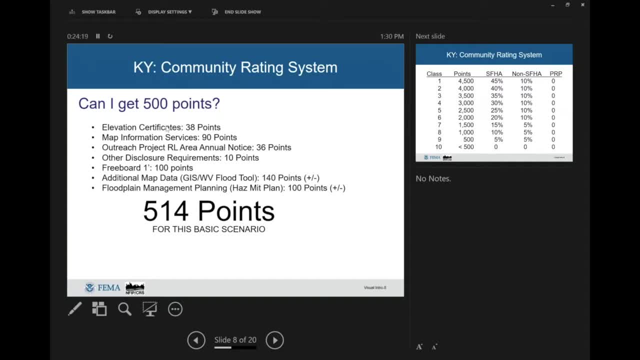 portal and find out. maybe the ground elevation in the particular spots 412 and the bfe in that particular same spot might be 415 and i can give those people that information and then they can know that, estimated, that in a hundred year event that they might have three foot of water to deal. 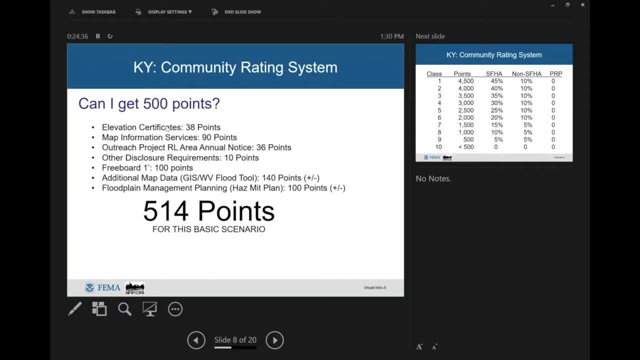 with now again estimates, and this is loose information, but it's better than knowing nothing at all, in our opinion. so we want to reward you for providing that kind of information and documenting with a log that you keep that information etc. and give 90 points there. um, most all communities have at. 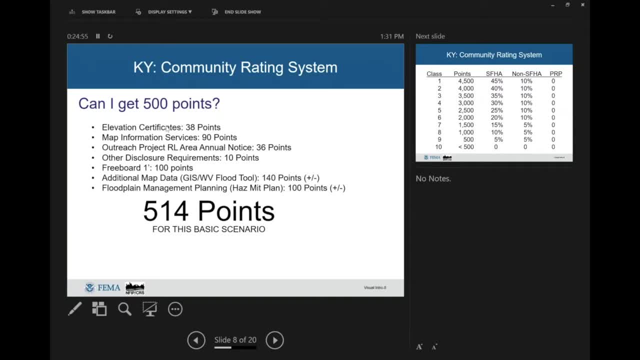 least one repetitive loss. so you're going to be required to send an annual outreach out to them that we can help you develop. but if you do that correctly, you could get 36 points under activity 330 for that annual outreach that you're required to send. so, um, that would be the 36. the other 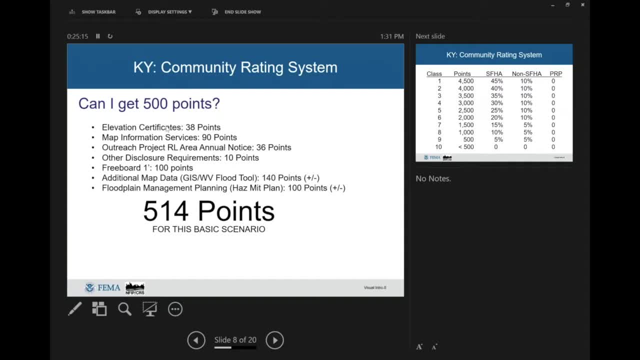 disclosure requirements are for real estate disclosures that are required by the state and also provide that the description of the floodplain hazard area being on the plat, as i was describing at the beginning of the session, that could get 10 points if i had one foot of freeboard. i could get 100 points if i searched my gis data using the state or my local. 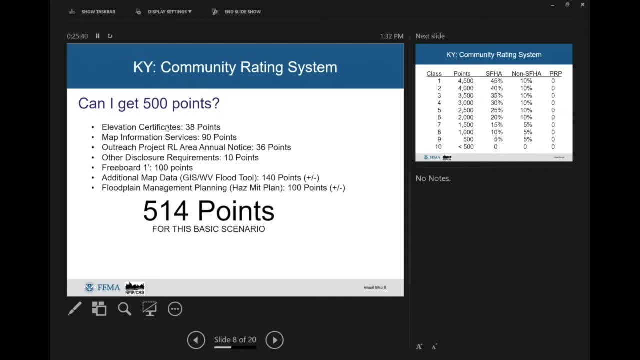 tool, or even the one my assessor's office has, and this doesn't have to be on gis, it's worth noting. it does not have to be available to the public, it has to be available for in-office use, so it doesn't have to be on a portal. that i would. 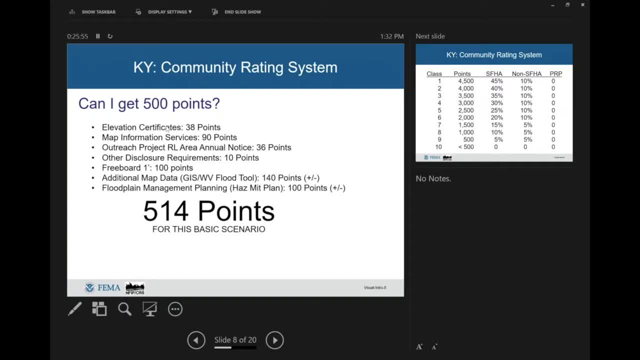 log on to or a website, but as long as you're using it and helping make decisions and also give out information, so it would be the best available data to you. um, we would reward that credit and it's about 140 points. there are additional points in that category, but i'm trying. 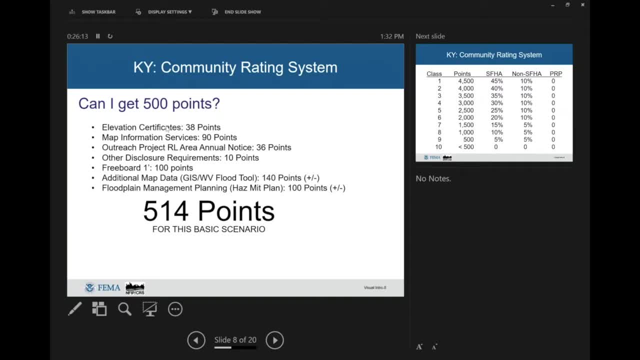 to kind of keep with the low hanging fruit. to show you guys, there are 500 points sitting out there: the floodplain management plan which, like i talked about, your multi-hazard mitigation plan. if that's been something that you participated in, you could probably very easily 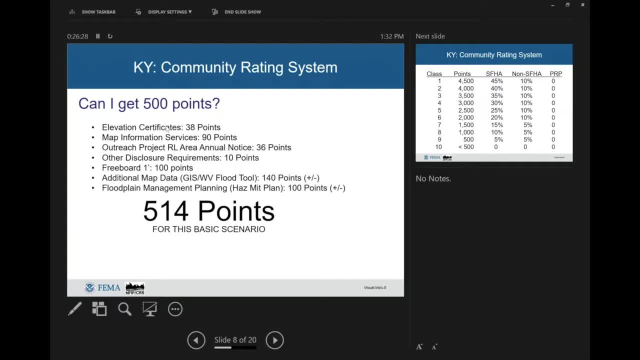 realize 100 points for that, and we would be able to then, in this scenario, have 514 points. now there are a couple forms that require signatures. we got to have some conversations that'd be like a little interview, this. it doesn't go without any work at all, but i think what i'm trying 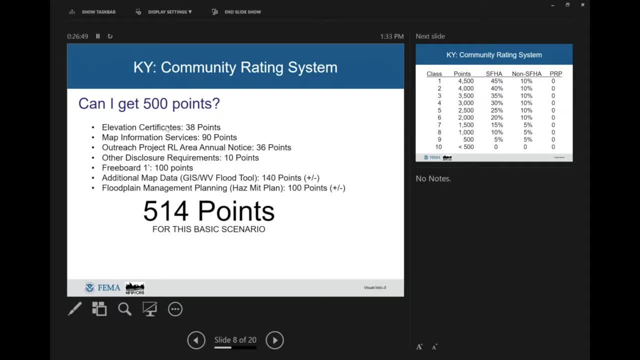 to say for you guys is: the 500 points is out there without probably your community spending any additional monies. uh, probably your community making you dedicate time to create new things or new activities. um, there's low hanging fruit out there by the resources put out by the state. 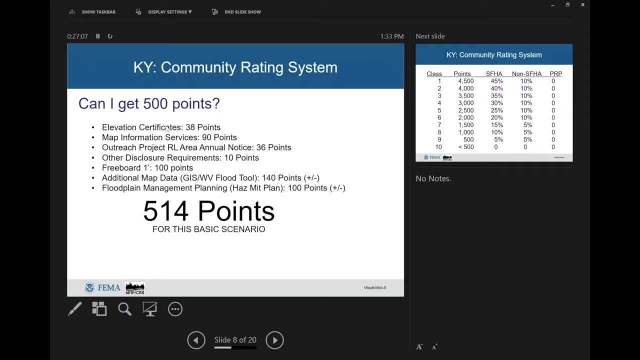 and by your communities that you could take credit for and probably realize a five percent discount on your flood insurance in those communities. so we um want to. we want to see communities take advantage of those things because they are there and we hope that with those lower rates that more people would take the policy out to protect. 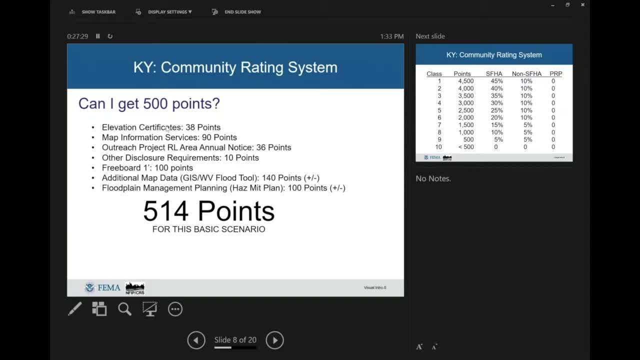 themselves, which only makes your community stronger. so before you move on, i just want to remind everybody guys, if you have questions as we're going through, please send them to me in that chat so i can collect them and have christina answer for you guys at the end. 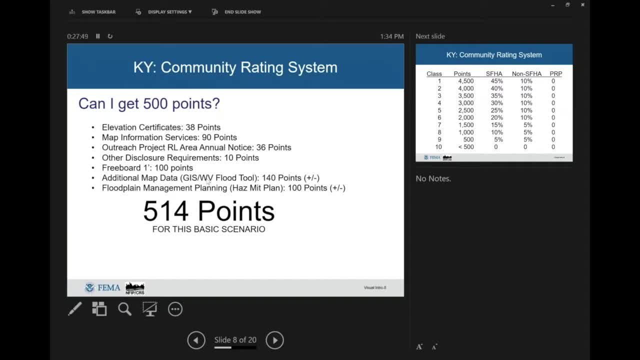 yes, and that's actually, and i want to point out- i'm so sorry guys, i give a similar. i gave a similar presentation. if you see where my mouth is, that says wv. it should be the ky flood tool. west virginia has a flood tool as well and i just did something similar from them. 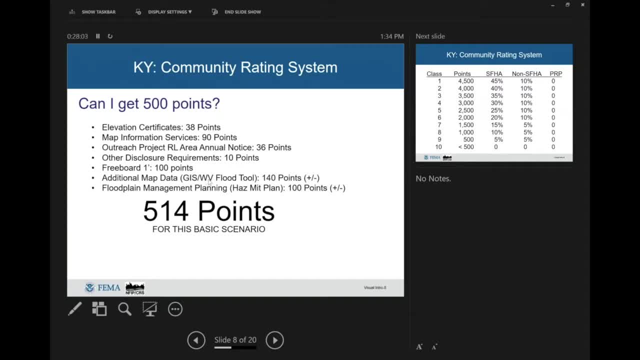 a couple months ago, so overlook that. i will update that, alex, before i give you the presentation. um, but it should be the kentucky. it's the risk map portal tool is what i was referring to. um, with all the layers for the communities that are credit worthy. 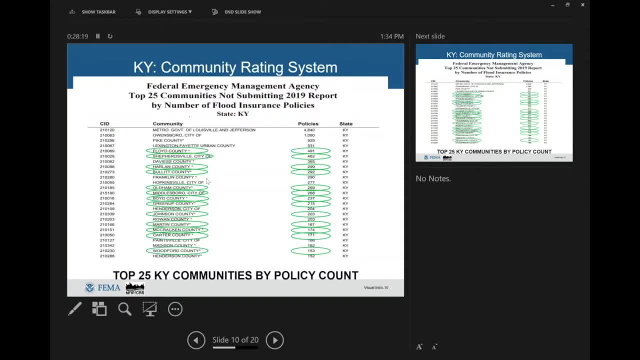 so, um, we looked at the point scale, um, and so i went through and looked at the top 25 communities by policy count and if you're circled in green, that means you're in the top 25 by policy in the state of kentucky and you're not in the crs program. perhaps i should have circled you in red instead. 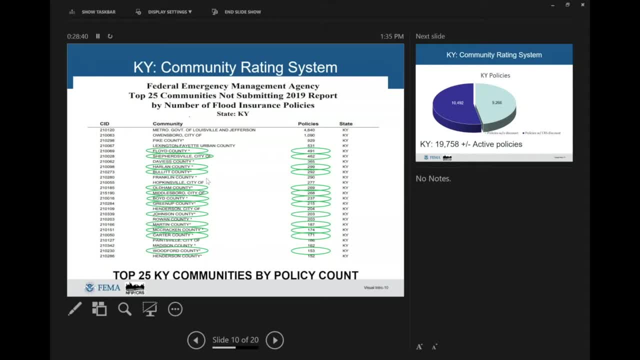 but we did green. so green meaning go like you should be trying to talk to alex to find out if you could get a cab, to find out if we could get you in the state of kentucky and you're not in the crs, um, but you can see that there are, you know, a couple thousand policies in the top 25 sitting. 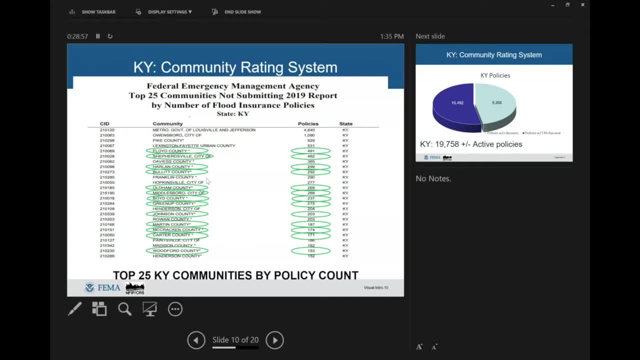 there getting no discount. and when you look at those top 25s cumulatively, so the ones not circled are already in. and then that brought the question to mind for me is how much of kentucky, uh, policy-wise, is getting a discount? um, so i was curious, alex, have you ever looked at that number? 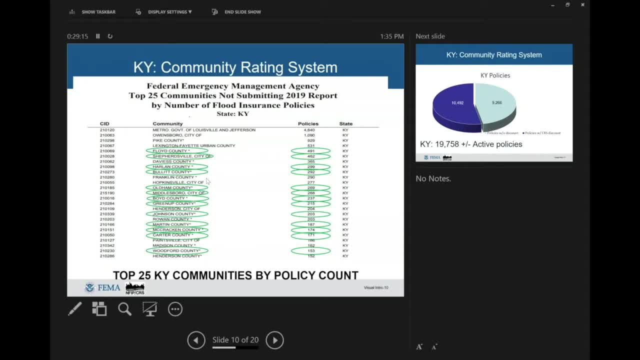 do you know what kentucky's is? i've got it on the next slide, but it's going to be on the next slide. it really made me wonder. i had to pull that information up today. all right, say that again. i'm sorry. i was asking if you had looked at kentucky's policy count. 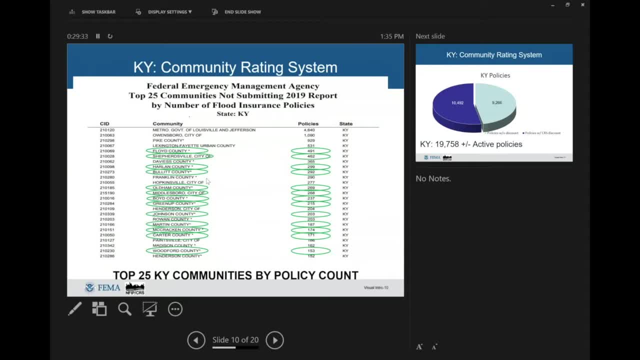 to ever see if, um, if we, if you knew how many were not getting a discount versus getting a discount in the state. i went and pulled that data this morning and i was kind of shocked by, um, how many were letting get by with our opportunity. we're going to, i'm going to have to. 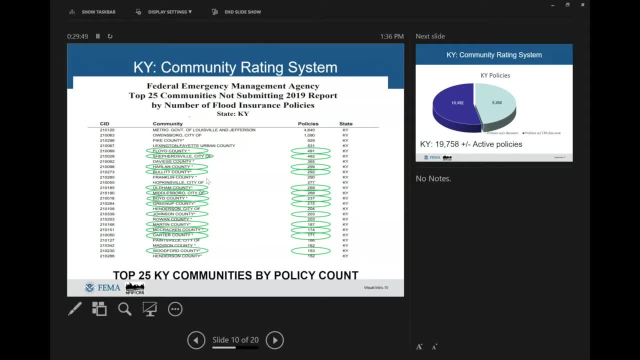 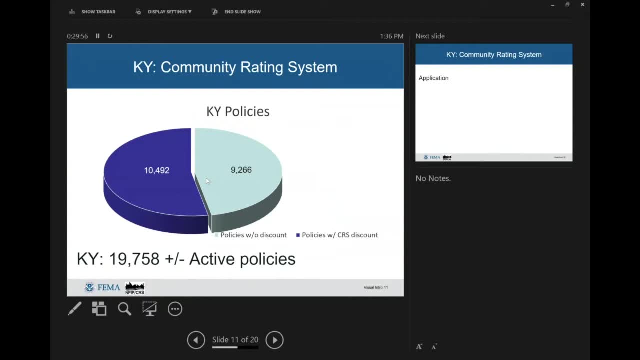 harass a few more people to get discounts. alex, yeah, i'm not sure, uh, what the breakdown is between those i know, prs communities. it's. the average savings is 88 per policy, but as far as how many are getting it, i don't know. yeah, so i went through and did the math this morning because i really 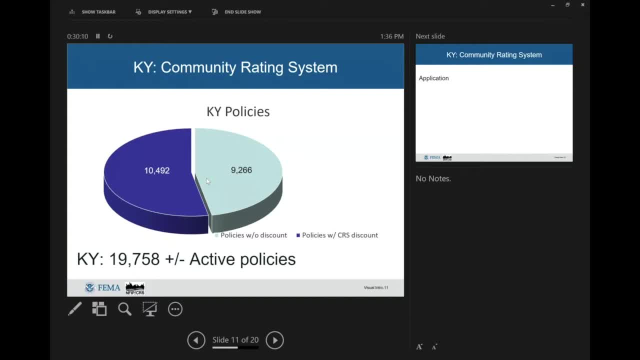 thought that was a good question to talk about today. and we're looking at cumulatively- we've got about nineteen thousand seven hundred and fifty eight policy-wise and we're looking at how many policies per crs, cis, which. so for all of you guys listening, that means that you know that's. 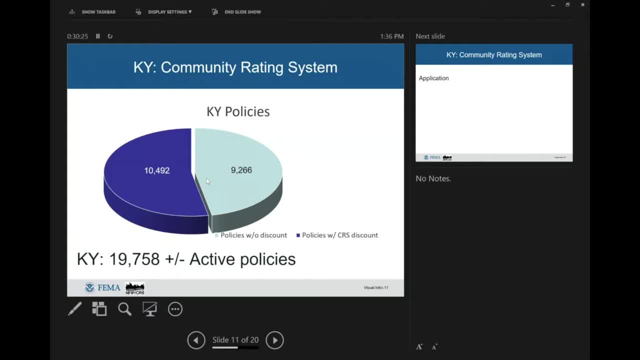 the database um for fema with that you know kind of gives us our stats on flood insurance. so it may be a month or two behind and that policy count total may fluctuate a little bit but let's say roughly we're just shy of 20 000 policies in the state um and you can see in the dark blue are the 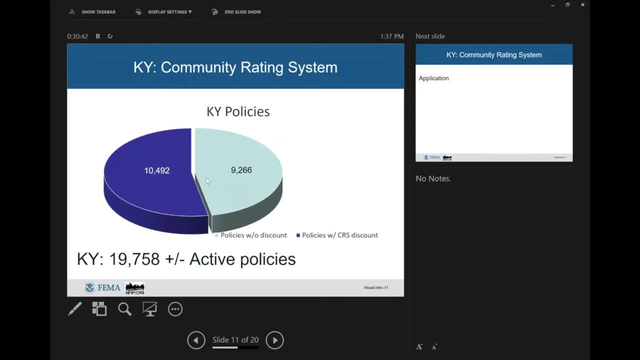 policies with the discount and in the light is the policies without. so we're looking at like right at the bottom right hand side of the screen. so we're looking at a little less than half of our policies are not getting a discount in the state of kentucky, so i think we need to get some more um. 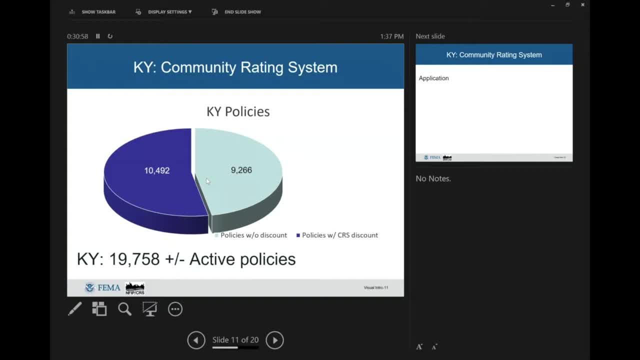 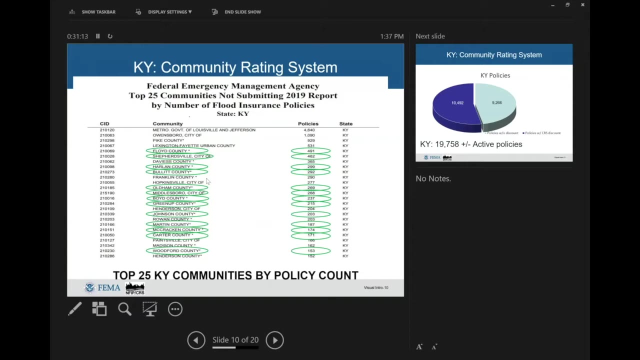 communities in, because those folks need to get discounts so we can encourage other people to continue to take flood insurance out. so 10 000 policies are are getting a discount, but we're still left with 9 000 not and, and then i'll revisit this list if you're, and i'll say that you. 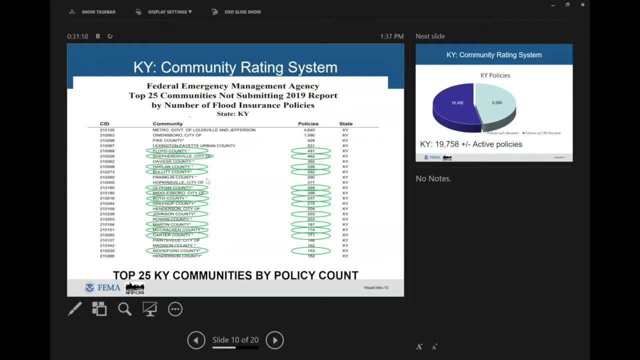 know, middles world owned on those communities, johnson county, um, which actually i'll plug johnson county to say i just heard from some folks from johnson county like yesterday, so, um, those are folks that we would love to talk to, obviously on the crs side, because what you're the 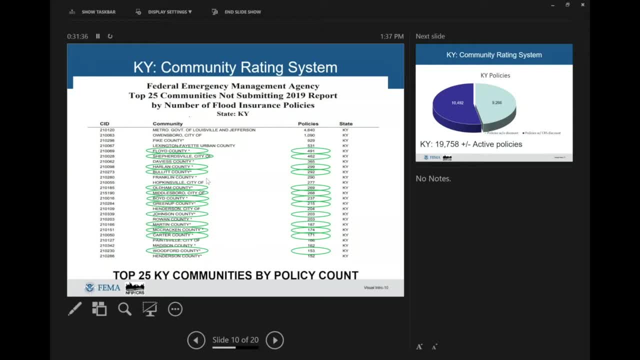 higher policy counts in this state. but, with that said, we have some communities- especially when they're like the county in multiple cities- that go through one agency, maybe the planning commission, such as pendleton county. brian thompson is the planning person in pendleton county and when he 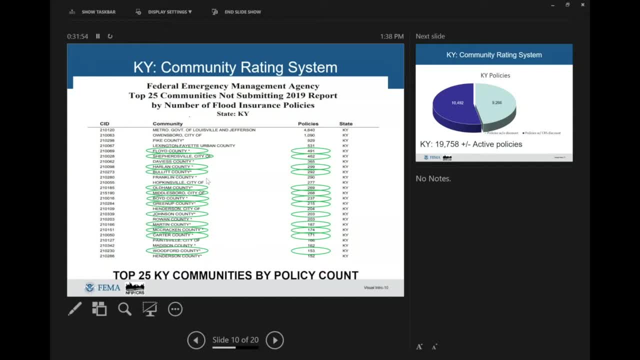 did the application for a couple communities that have higher policy counts. we went ahead and did it for all of them because he was going to manage all of their applications and even though they were maybe lower policy counts, they were able to get the benefit and it really created almost no. 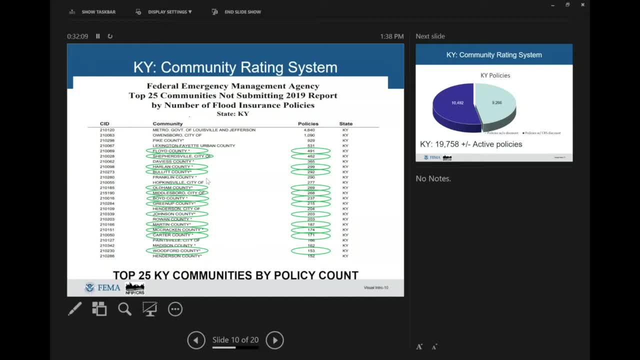 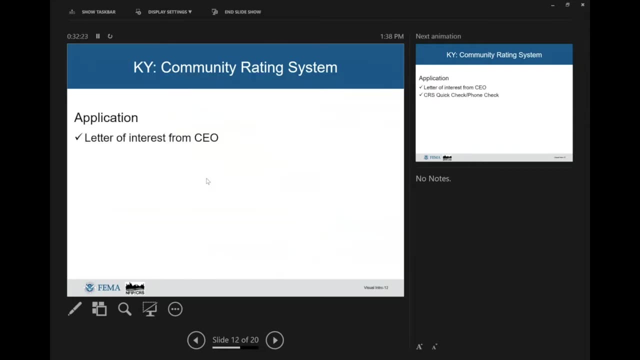 more work for brian because he's doing it all as a package deal. so certainly always keep in mind we can work with those things as well. um, Heidi, and then that last slide unanexed: um, okay, thank you. um a and um, down, down, down. 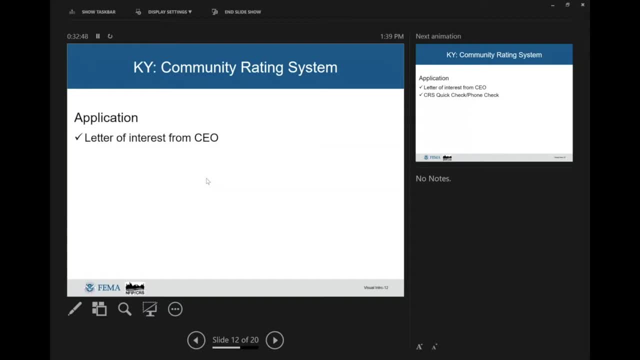 down program. so therefore, come and complete a cab. for me a community assistance, is it? you're asking Alex and the FEMA region folks to come and do a cab, look at your floodplain and check about. you know your permits that have been issued, what's been built and maybe Alex can do. you have a one or two sentence. go to Alex. 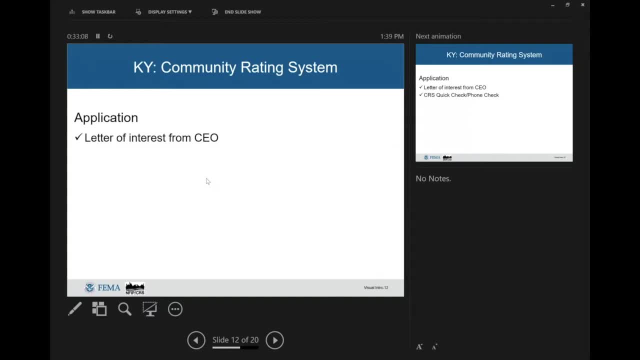 for what a cab is for them. yeah, so, essentially, guys, the easiest way to think about it, it's an assessment of your floodplain permitting program. so, are you issuing permits the way you're supposed to? are you regulating development the way you're supposed to? basically, I'm going to compare your. 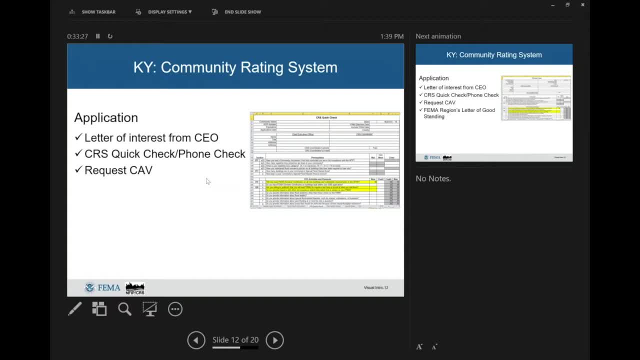 program to what we do at the state to make sure they match perfect. so once you have a clean cab is what we call it, or a good cab- they're going to give you what they call a letter of good standing. I like to say it's like getting their. 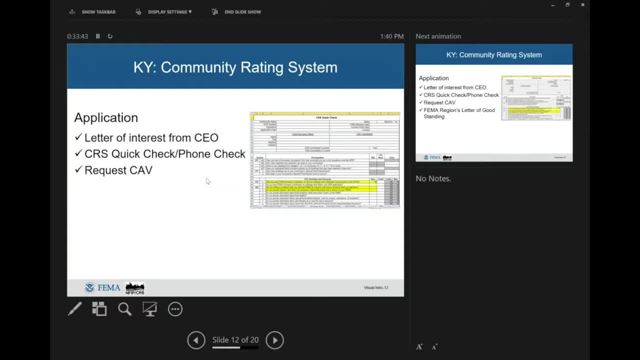 blessings like: so you can say they say you're all, you're great and we can put you into the CRS program at some point in that process. between the letter of interest in the cab, once that letter goes out, I'd like to either have myself or Alex have. 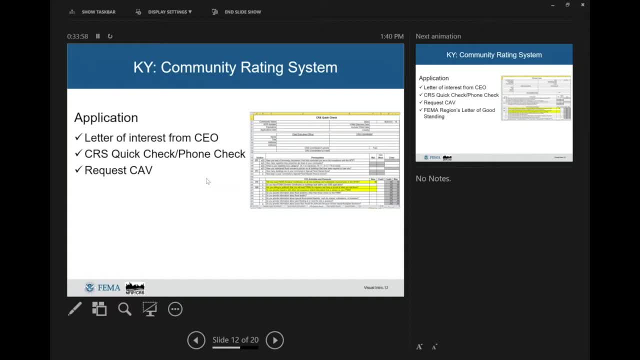 a phone call and just we want to do a drive-by. I want to know what your basic floodplain regulations are. I want to know that, if I haven't sat down with you at cam before and look at your ordinance, tell me if you have some free board or a. 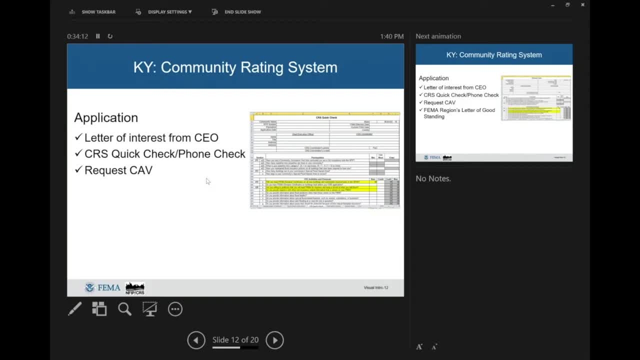 good example with Augusta. Kentucky wanted to join, which we were really glad to have them. they were wonderful to work with that. they had a case where they didn't have any free board in their ordinance, so that was a hundred points we couldn't collect. so we wanted to have a phone conversation to see what else they were doing. so we 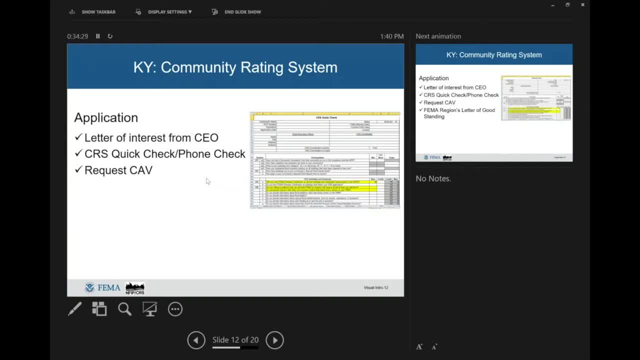 could make sure we could get to that 500 point mark, because there's no like 4% discount. you got to get to 500 and you know it's not prorated at all, and that call enabled us to see that they had really great staff there to work with in. 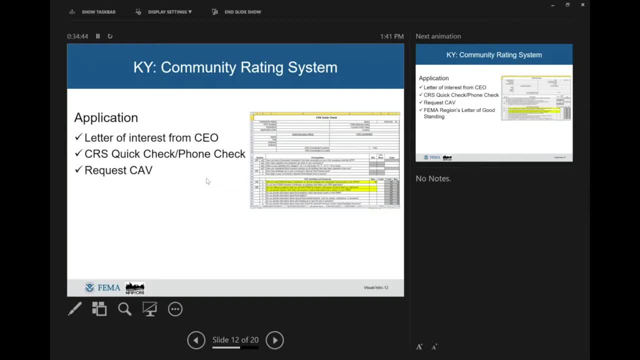 that we knew that they would document and that we could get them into the program even without the entire standards that some of our other opportunities have. that makes that chunk of points coming to play, and so we just want to have that call to see what we need to do, because if we do have the 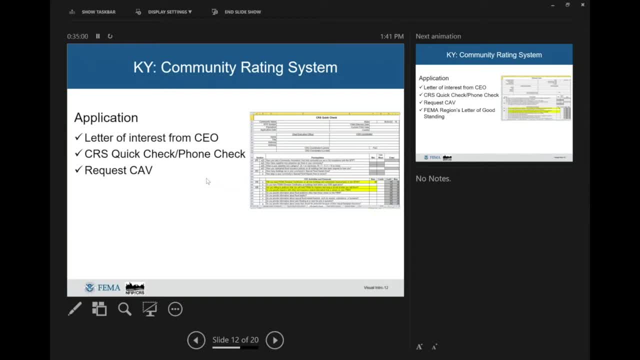 case set where there's absolutely no way to get to that minimum 500. we don't want to put you through the process, and so that's the letter. some point in time we have a phone call. you have your cav requested from that letter. by the way, he's asked me to continue as long as I can use this call, since we don't get a slow and good letter. 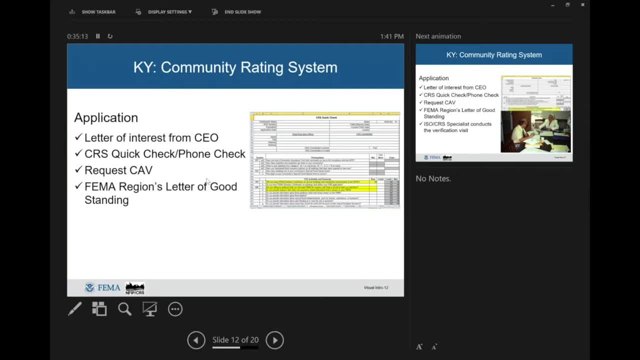 the letter we have a template of and I'll show you, guys, you don't have to write it blindly. and we have a template that says: hey, this is what we want, and you don't have to reinvent the wheel and once they issue the letter of good, 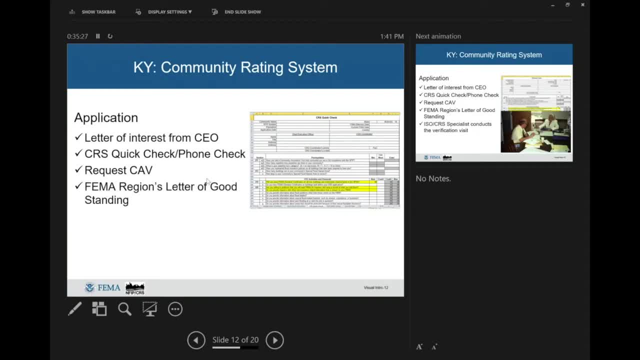 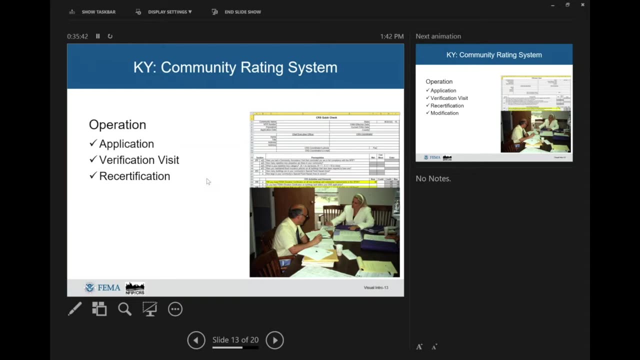 standing. then I went the wrong way, sorry, and the specialist myself will either do it via phone or in person. we'll do our verification with you and you're starting to roll. once you're in the program you have, you know your application was what we just described: your verification visit and then, once a 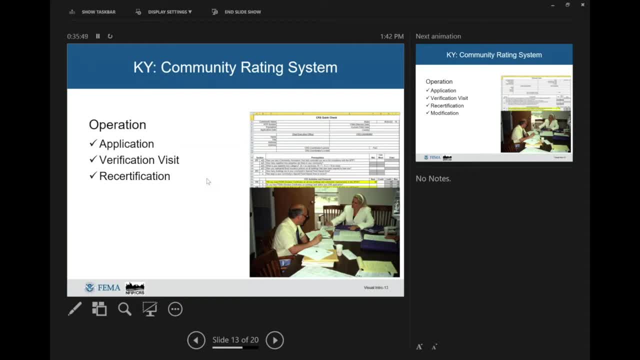 year we have something called a recertification. that recertification is done via email. it's a way to touch base with you. it's going to be a page that says: hey, here are a lot of statements that you get credit for, and if you don't? 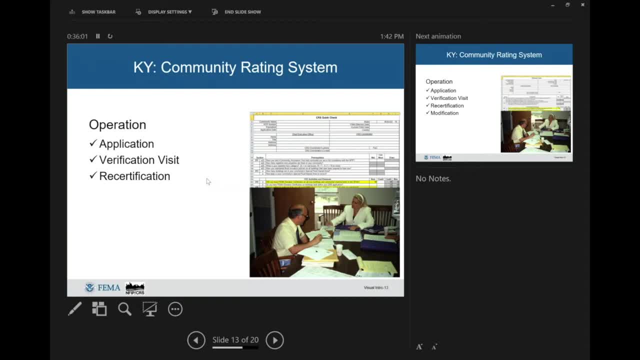 get credit for the statement won't be there. they're going to ask you to initial beside the statement saying, yes, we are still collecting elevation certificates, and they're going to tell you we want you to attach elevation certificates, or? yes, I am still writing the log down of people who ask me about M I enter out of the floodplain. 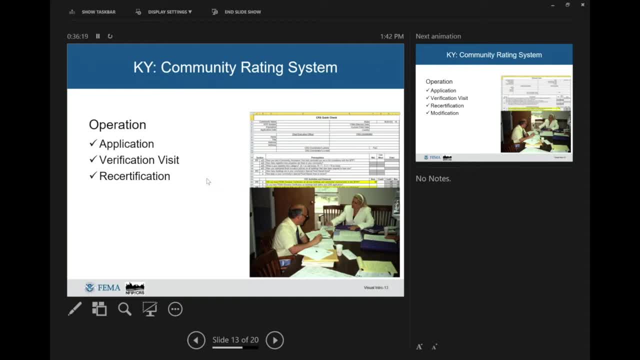 and they might ask you to attach a copy of the last years log- and not everything asks for an attachment. it'll tell you what it wants and then you just email it back. you get about 45 days to do that pretty simple process. it's just a way of. verifying, because otherwise we only see you once every five years. if you're a, You're in between the five years and you do something great like I described with the city of Richmond and you increase your standards and you want to realize that we can do what we call a modification, where we're just looking at the credit you want to get more points for and we don't go through the whole process all over again. 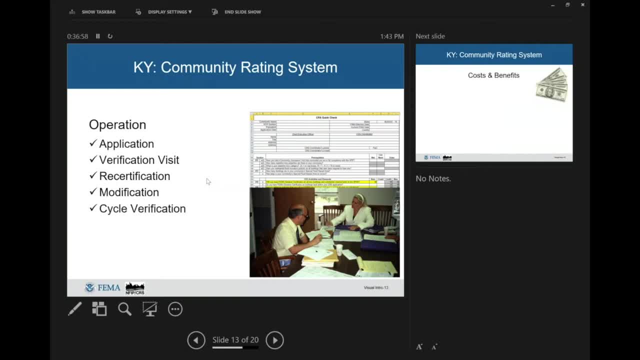 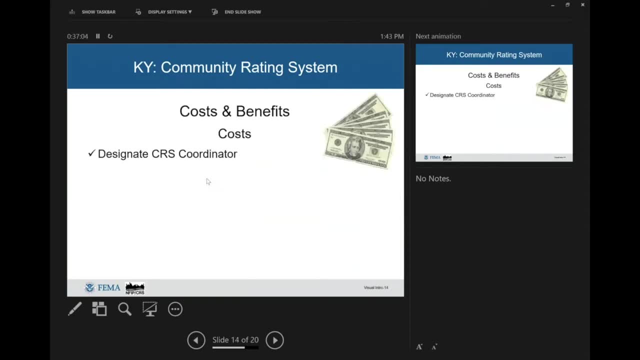 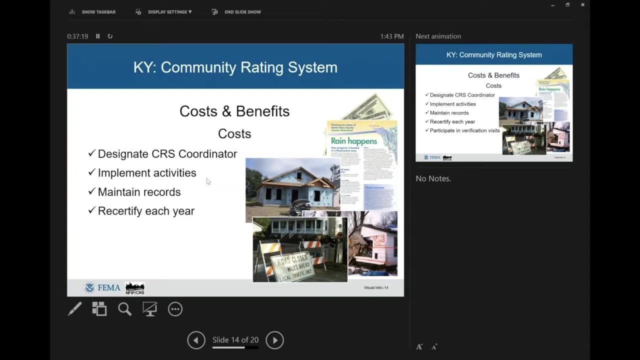 And we can then get you more credit and a better discount. So after all that again on the fifth year we come and visit you again, Or when they do it via phone, but most of the time we come in person. Benefits cost to this program is: you designate a CRS coordinator, you implement your activities, you keep your records up, go through the recertification, participate in the program. 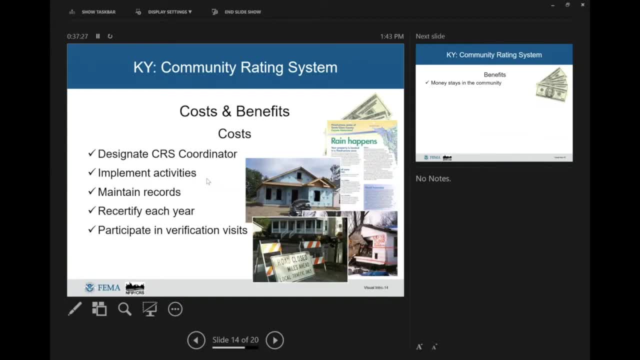 That's the cost. It's really all staff time. There's no monetary fee for participating. It is probably the only federal program that you're going to get into. You're going to get $50 back into the pocket of people that live, reside and vote in your community. 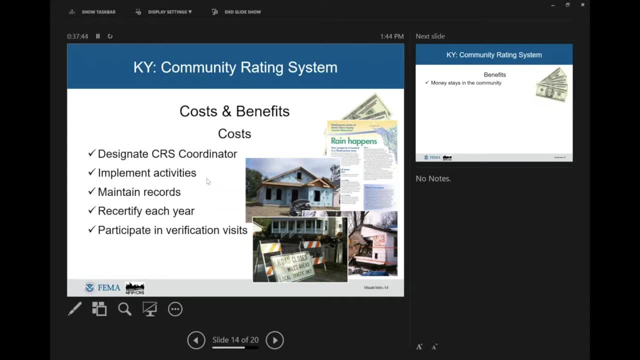 That's what I always like to remind our elected officials of- Probably not going to find too many else. Like Alex was describing, the average policy savings in the state of Kentucky is $88 a year. I find that often those people who get that savings and have that blood insurance policy more often than not for the masses- are people who really need to save that policy moneys. 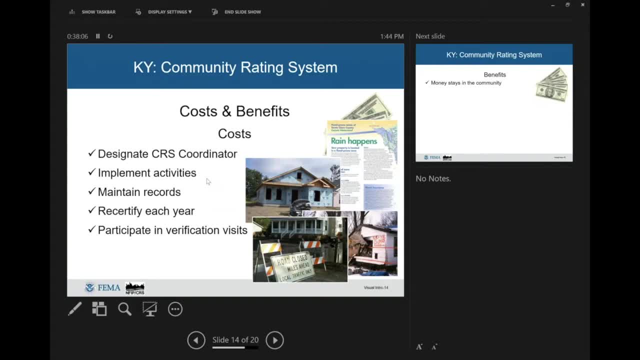 I was in one Kentucky community not long ago and we were in the field looking at a structure and the person told me that they were glad that and they described their savings as two water bills in a year. And I was like that person appreciates what their community was doing for them. 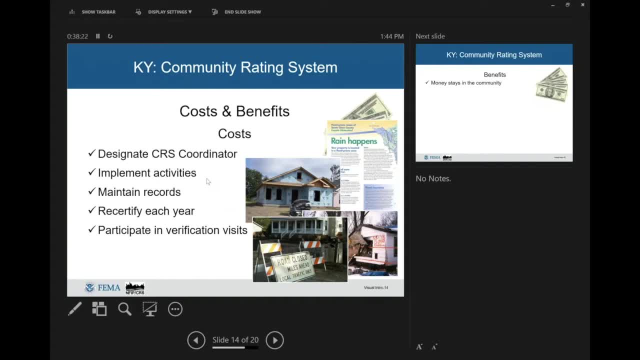 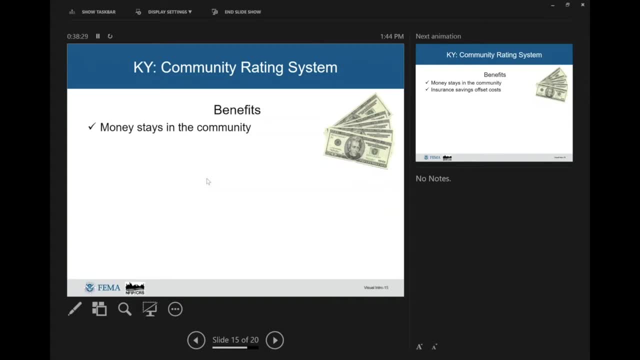 Because for those folks, they care about that discount and that savings. $88 was a lot to that person. So, but you don't pay a fee as a community. It's just the time that your staff is investing The benefits. 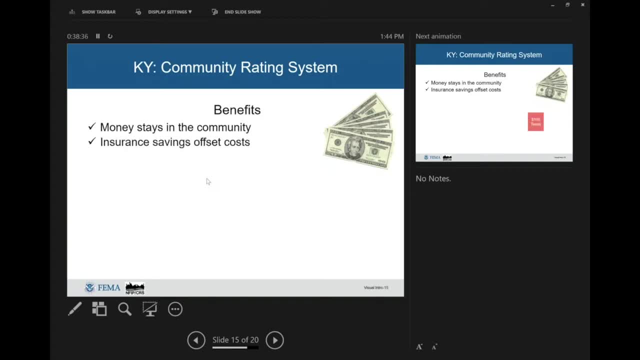 The money stays in The community. We hope that the savings to the people holding the policy and when they reinvest that money in the community it might offset the cost of your time that the community incurs Bitter. it builds better organized programs really. 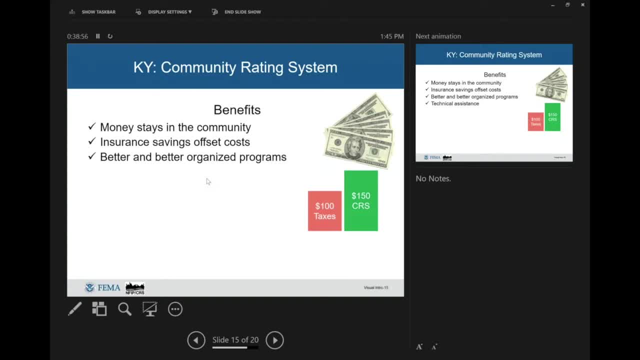 You know. so technical assistance is provided by myself as your CRS coordinator, by other places you'll see. You'll have WebEx. There's a lot of resources out there And other things available to you: Public information, really the consistency of getting out that public information, et cetera. that builds a lot of continuity in your floodplain management program, which makes it stronger, educates folks. 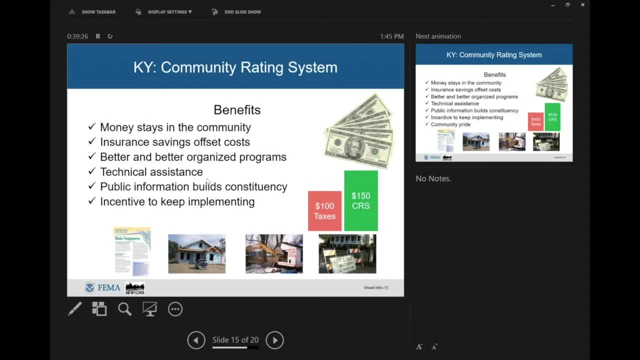 And it becomes an incentive to keep implementing. Like I said, most communities, once they get started, they want to do better and they keep looking for ways to do better Because they want to continue to stay, They want to continue to save the dollars. 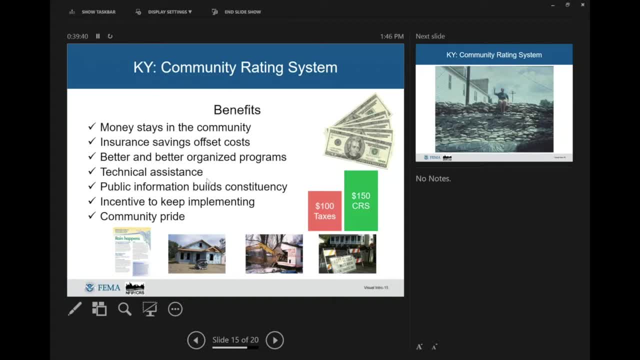 So it's a positive impact For my communities that probably have the most pride, have the fewest policies. I find that, like I know that, my little wolves of the world, my Birmingham, Alabamas- you know my bigger communities, I have a lot of larger metro areas. 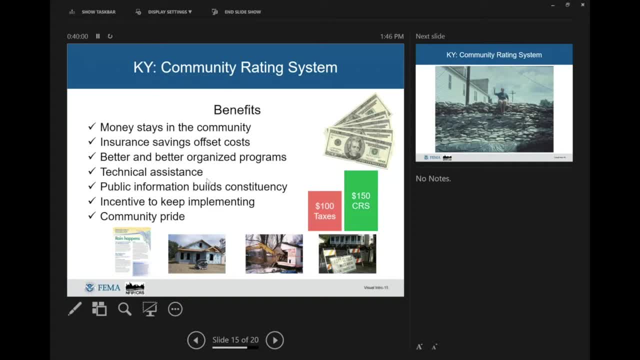 They are proud of their programs, no doubt, But I would challenge them to the pride of any of my two or three or four. I would challenge them to the pride of any of my two or three or four Because sometimes when I go to the place that has 53 policies, they are the ones that actually have people come in the door and tell them they're glad their flood insurance rates dropped. 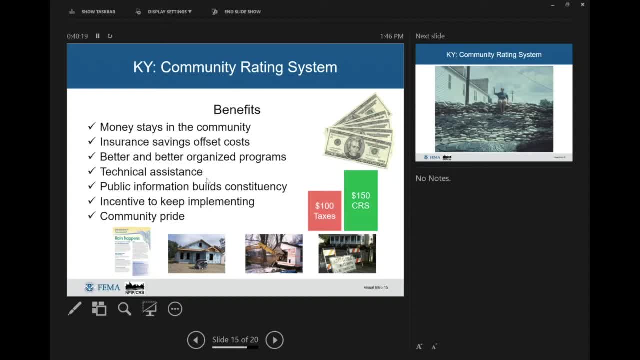 Because they have that small town relationship. I hear a lot from people that say that this is a program for a large city or a bigger community, And I really don't think that this is a program for any one particular size. I think a small community has just as much shot at. 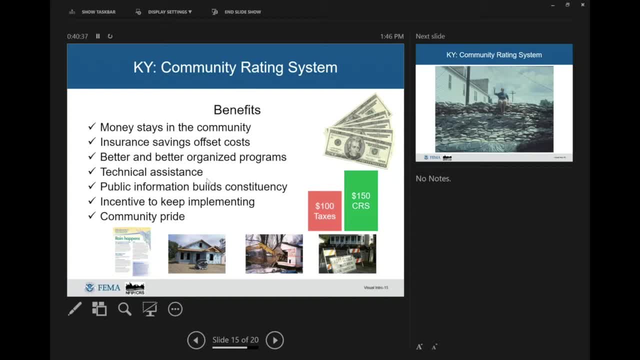 And being successful as a large one. Sometimes, I think, a small community even more so, because maybe what they have is a little more manageable. It's just that they educate themselves on the program along the way and build it up. I think the smaller jurisdictions stand the best chance for success in my planning floodplain management experience. 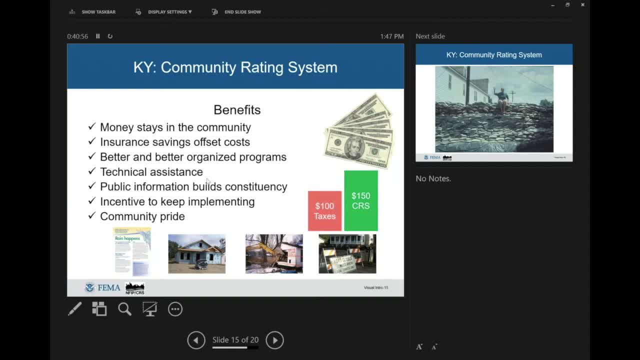 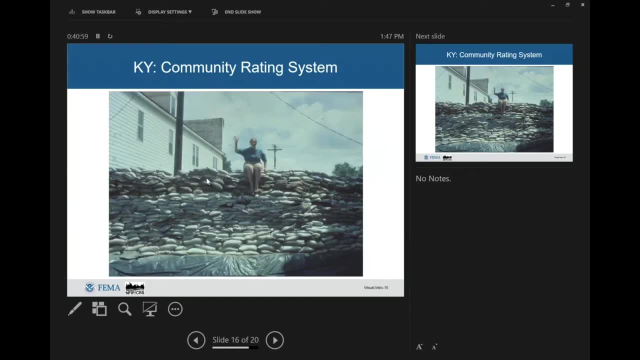 And now, having looked at it through the goggles of a specialist administering the program. So you know you get a lot of help. And I'm just going to put this in the chat. I'm going to pull up the list here We have the specialist, we have the state, FEMA region. 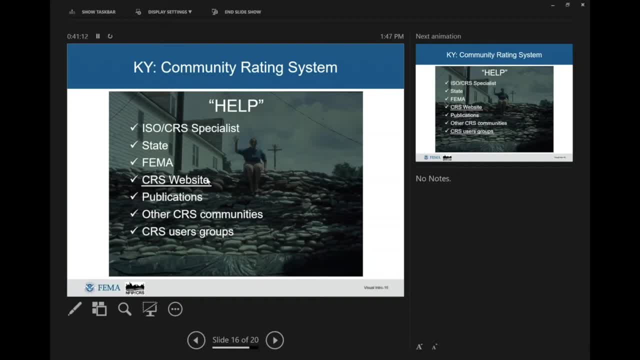 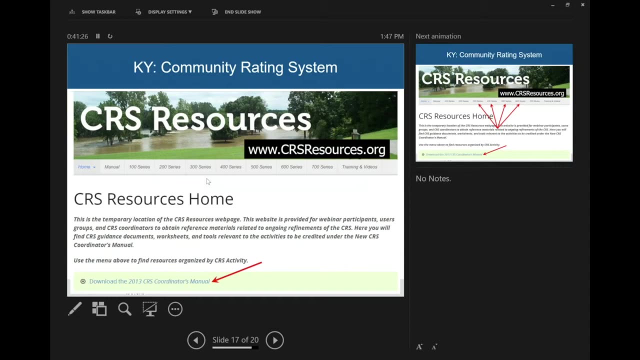 We have lots of publications on it. We continuously put out new things. but we have this really great website called CRSresourcesorg And I'm going to pull that up here. This is what it looks like And you can see. at the top of the website or on the website. you can download the manual. 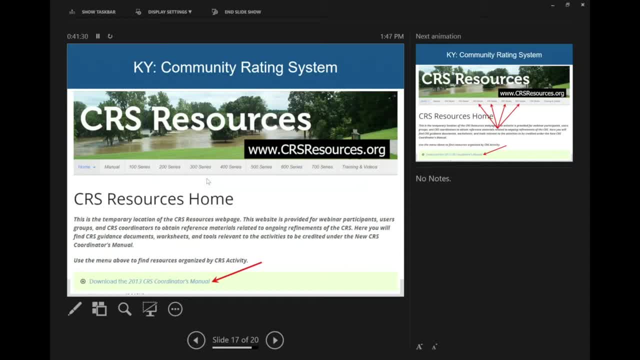 And, of course, that says the 2020 manual now or 2017 manual. But then if you go to the top, every tab has a list, Every tab has drop downs that then, when we talked about 310,, 320, 330, those numbered elements- they further drop down to show you those numbered elements. 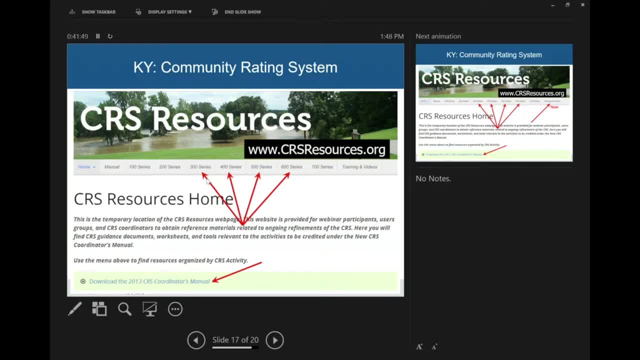 So when I talked about in 320 for map information service and that you would keep a log, well, those same, the same log that you would keep. example of that log is under this 300 tab, under 320.. And it's an Excel spreadsheet that says: you know, if you want to keep a log, you have to keep a log. 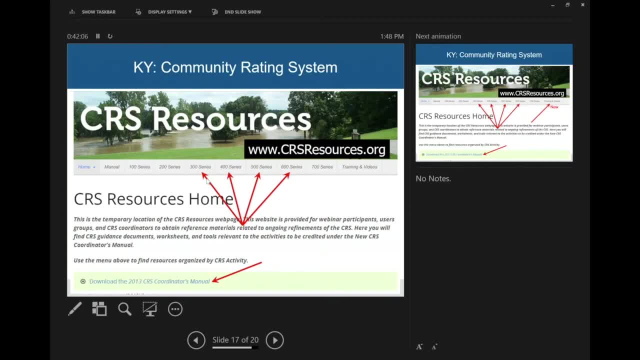 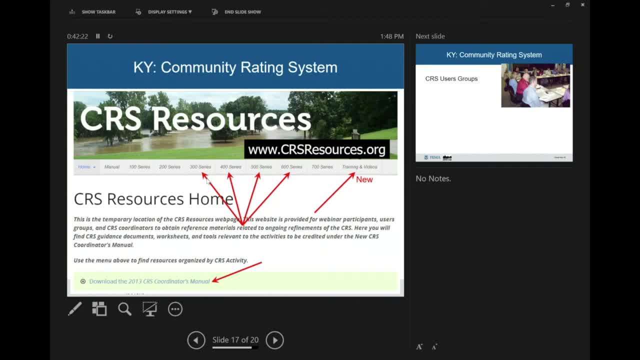 The last tab is training and videos, And there's always new content going up, but there's lots of live trainings. There's recorded trainings on specific activities, on general topics, And so we encourage everyone to visit the training And videos frequently. I know that Cam and Pam is really really great about sending out notices to remind people that training opportunities are coming up, especially when it comes to CRS. they're just super diligent about it. 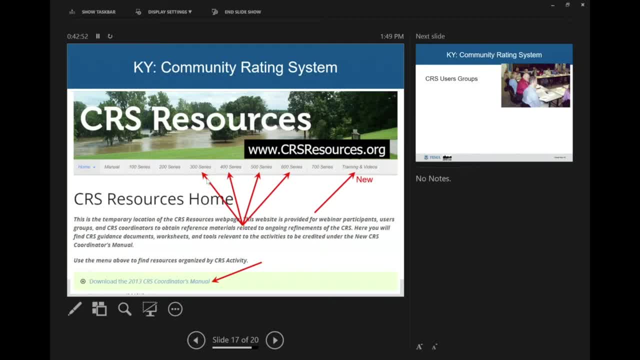 And so if you don't get her newsletters or email their notices, please reach out to them and sign up, because that's another reminder of CRS educational opportunities that are out there. And if you don't get her newsletters or email their notices, please reach out to them and sign up, because that's another reminder of CRS educational opportunities that are out there. 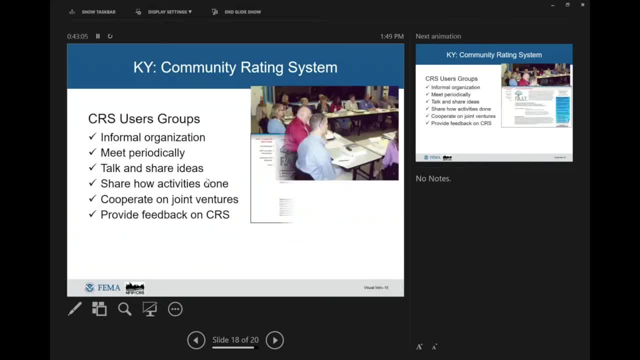 And so if you don't get her newsletters or email their notices, please reach out to them and sign up, because that's another reminder of CRS educational opportunities that are out there. There are users, groups, and I'm going to pull all these up so we can kind of continue on through time. 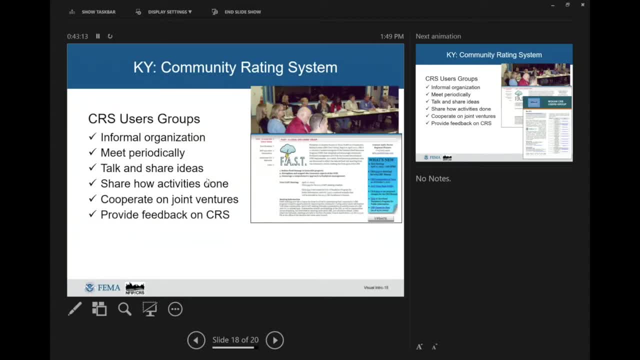 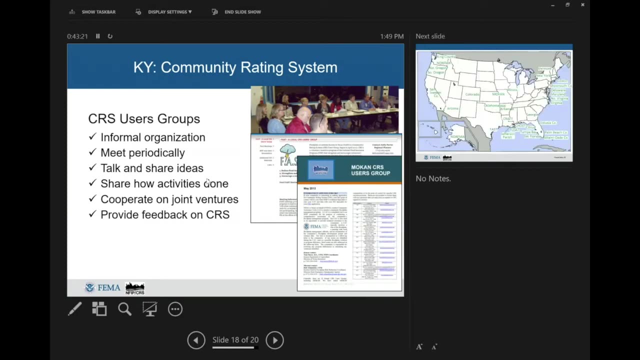 They're informal. They help each other grow. Kentucky has one being cultivated. The idea is to learn from each other, utilize resources from each other. You can see they're kind of popping up all over the country. The coastal areas have kind of already been saturated with users groups and we're seeing those more and more now in the inland areas. 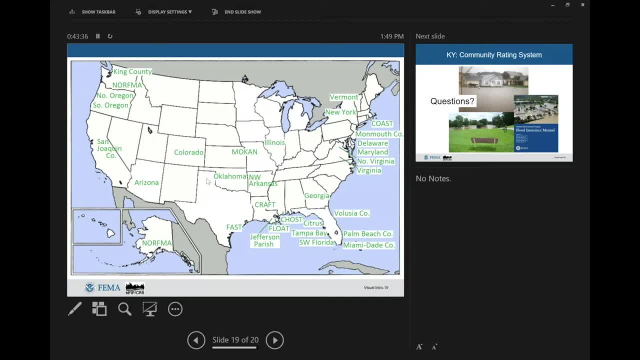 West Virginia started one. Tennessee now has one. They're not waiting on FEMA to give us an updated map on this, but Tennessee and West Virginia are two of the new ones as well, So you'll have those as resources. I actually tell everyone- the MOCAN, the one at Missouri and Kansas out in the middle- their website's really good. 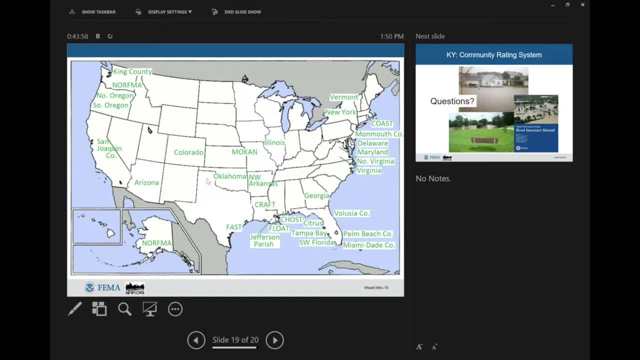 And while they're coastal- the one here in Virginia on the coast- they are a really good one too, With a really great website. they have lots of resources and not all of it's coastal, So therefore you can- and they record their user group meetings and put them on there so you can always go back and learn about things through them. 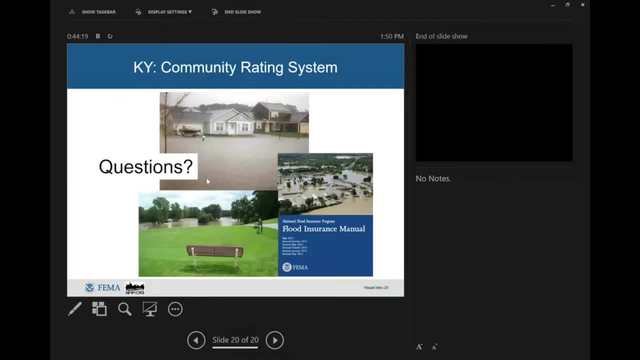 So a lot of good resources out there, And at this juncture I will. I'm going to insert one thing before I go to questions. With the CRS program, there are two times a year that new communities or existing communities can change a discount. 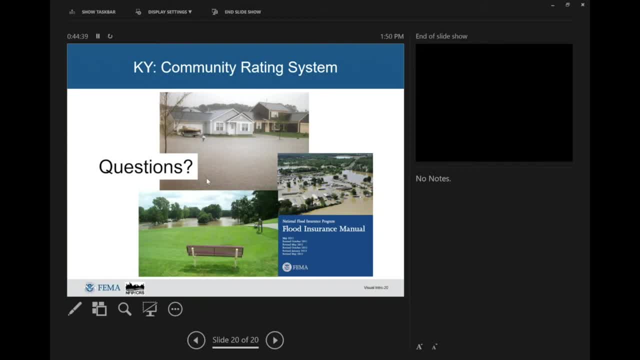 So if you're new, you're a Class 10 with no discount, and maybe you get your application in and you're going to be an 8.. Only on May 1st and October 1st do those discount changes take effect on the flood insurance manual published by FEMA. 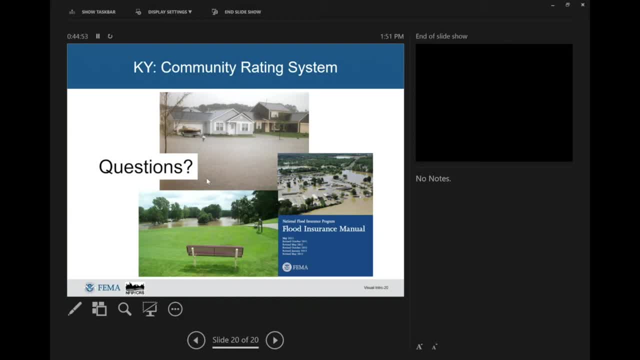 So there is a lead-in process. I want to remind folks that it's not a fast process. We have certainly turned over some pretty fast applications for new communities and we've been really proud of that with Kentucky We've had it to where we've been given letters of good standing, and Alex has worked diligently and got communities ready to go. 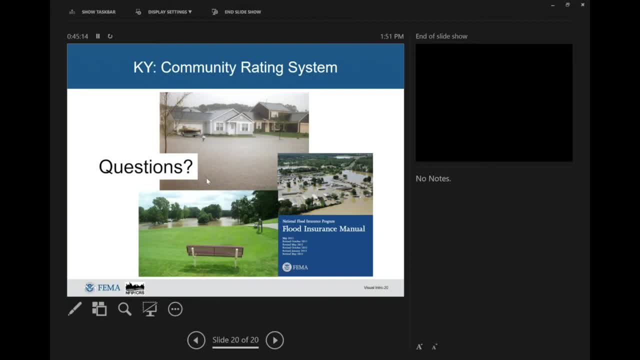 And I, you know, got that letter and we were able, out of the gate, to work with them And they were willing to step up to the plate with dedicating a little bit of time and said: let's get our application in so we can make the very next effective list, because there's about a six-month lead time on those effective lists. 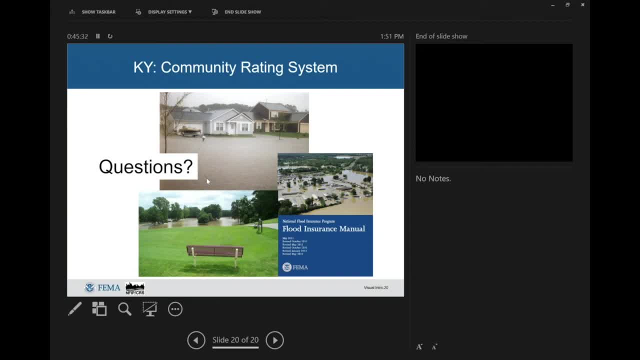 So on October's list, it usually goes in by- excuse me- in April. so if that gives you an idea like so, from April to October, it's dead. nobody gets added to it. That list is being processed at headquarters for the insurance manual. 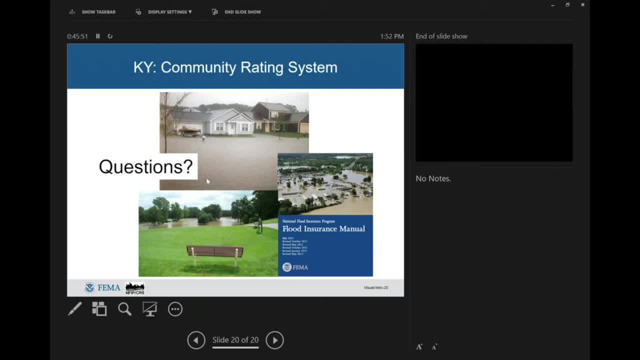 So there are lead times and if you're thinking of doing this, you know definitely reach out. You can never start having the conversation with us too early so we can help you guys plan your timeline And it's not a surprise later saying, oh, we want to join. 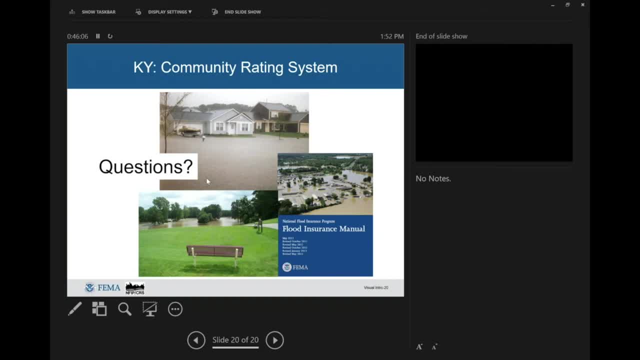 But we didn't realize it was going to take us nine months to realize our first discount on a bill. And that discount it is printed on the bill. actually It says Alex Van Pelt's flood insurance is $1,000 a year and his community has got a Class 8 rating. we're seeing a 10% discount. 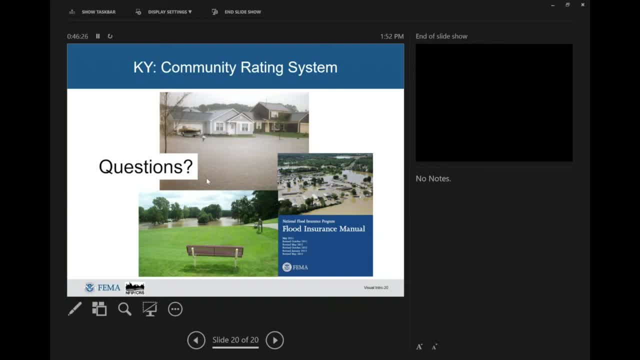 So therefore, he's getting $100 off his bill and his new total is $900.. So these people actually do get it in hand. It's something that they see that you, as a community, that you're doing and helping them and, like I said, 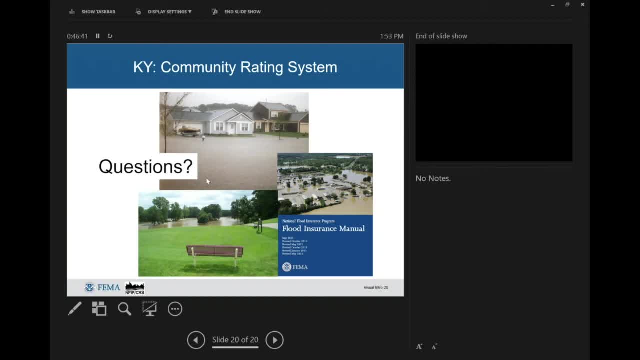 putting dollars back into their pockets and into your community. So that is CRS in an intro nutshell. It is a big program. It is that we have a lot of resources here, so it doesn't have to be a burden at all. It can be a very, very positive thing for your community. 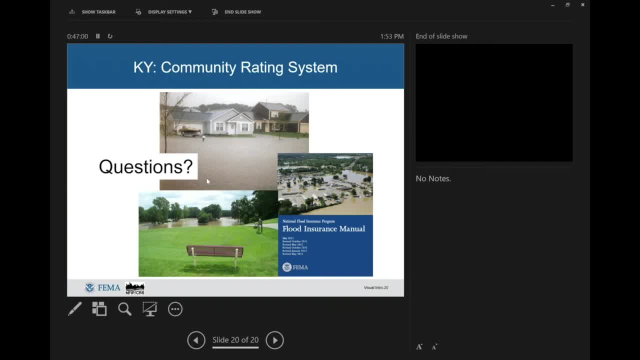 And with that said, I'm going to turn it over to Alex. Yeah, Thanks guys. Guys, if you still have questions, go ahead and send them in using that chat box. I'm still here, I'm still taking them. 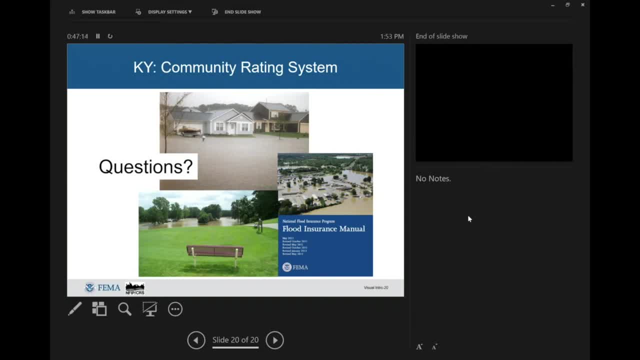 Christina, I do have a couple- I guess I might call them- softball questions that you kind of touched on, but I want you to go back and maybe touch on it a little more in depth, if you don't mind, Absolutely. So the first one is: you talk about some of the different activities that were out there. 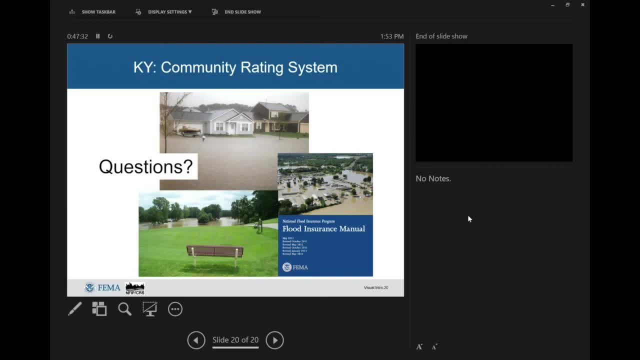 the elevation certificates and the mapping information, things like that. So the question is: do I have to do all of the activities that you listed? Can I do only some of them? Who gets to choose what activities are done? Absolutely Great question. So it is an a la carte program. The only things required. 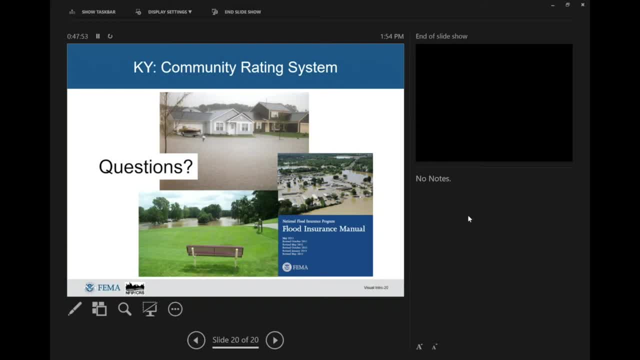 of you are what we call the program data table, which means you have to tell us how many acres of 100-year floodplain you have and how many buildings are in the hundred. how many insurable buildings, let me say, are in that hundred year? Now, don't let that scare you away. 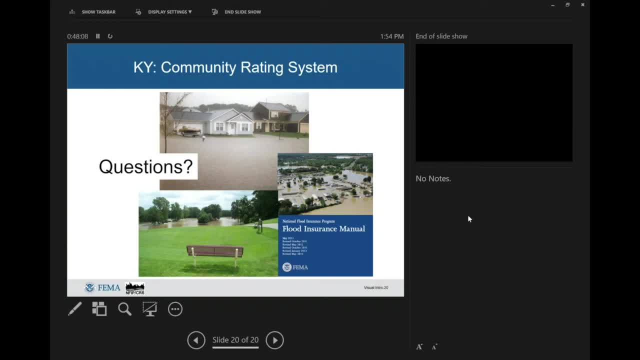 because if you don't have those capabilities in-house, we have had super success with Anne-Marie and Carrie and the folks there calculating that within like I mean literally. sometimes it's in minutes, they're so fast If you don't have GIS in-house and those capabilities we can get. 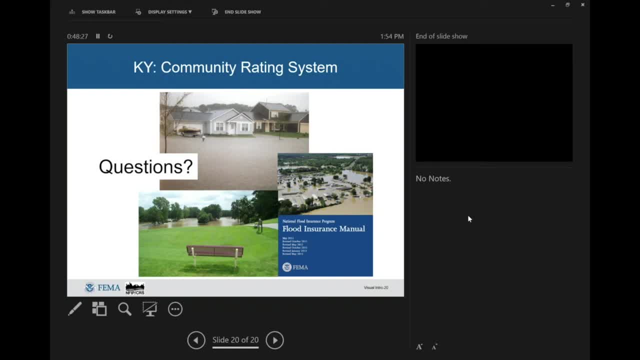 that for you. Second, you're required to do elevation certificates. That is a requirement, And the next, only other requirement in this program is for repetitive loss, depending on how many you have. I know the masses of Kentucky have probably less than 50, which would just mean. 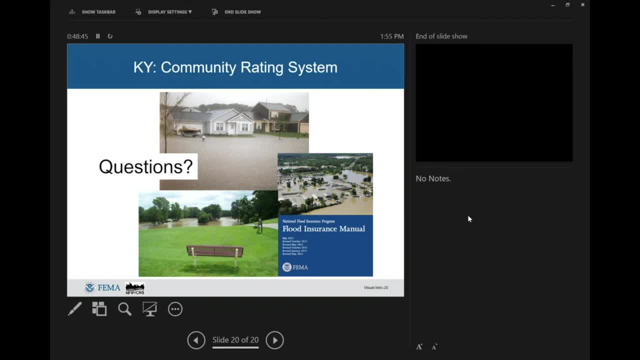 that if it's an outreach and we have to do some mapping work on it and identify the areas, which is something we walk you through and will help you build your outreach. Those are the only three requirements. Everything else is a la carte in this program. If you have. 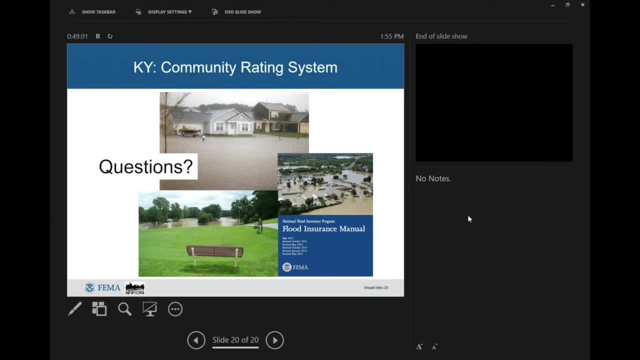 four foot of freeboard and you have a hazard mitigation plan. you're going to have to do it within a day. It's not a good idea to take those three minutes and you're going to be out of time, So you're going to have to do something that will help you with that. 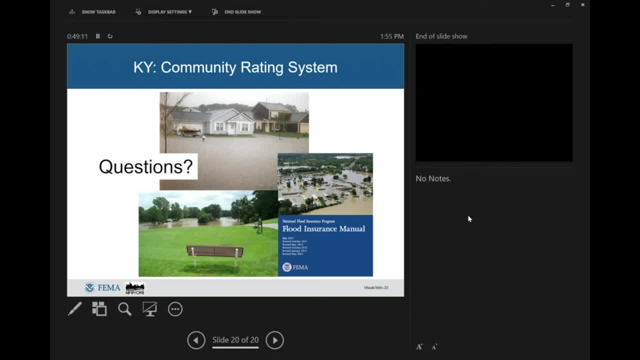 And you're also going to have to be a little bit faster in your navigation plan. As long as you do those other three things I just named, That could get you 500 points and you wouldn't have to touch anything else, so to speak. So does that answer your question, Alex? 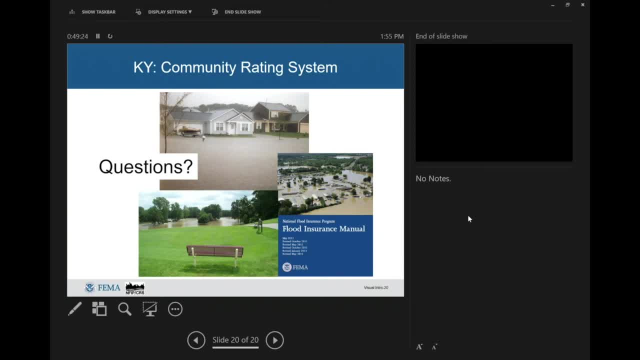 Yeah, that's exactly what I was wanting to touch on is the a la carte part. The other question, yeah, the other question we had was who is the CRS coordinator in the community? Is there a single person that should take the lead? Can anybody do it? Is somebody's job duty, like how to do it, how to do it. 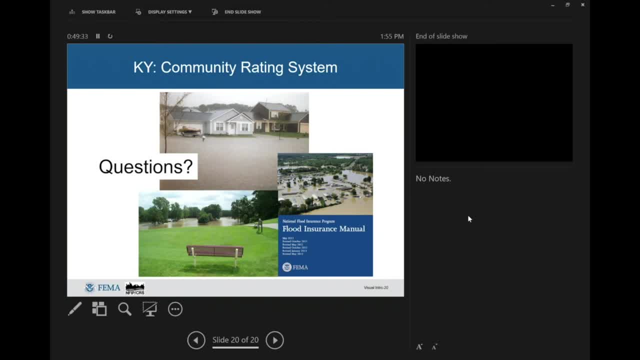 job duties. like how does that work? absolutely good question too. that's really good. um, so it can be anybody in the community. um, for example, in um in one of my really small uh communities in west called watcher free, virginia, out on the coast, the mayor of the town, of 100 people, is the crs. 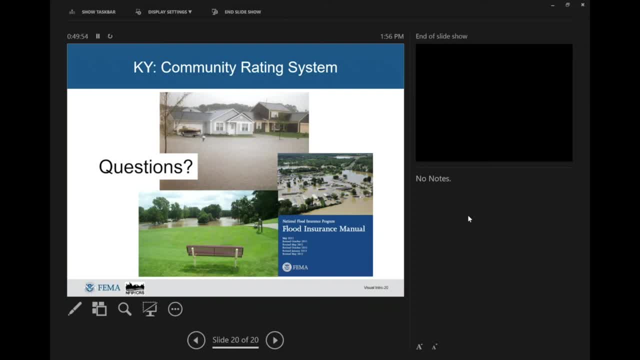 coordinator, um then it could be the planner, it could be absolutely anybody. they just decide and designate a crs coordinator and while it's not the most ideal, the crs coordinator does not have to be the flood expert, because what it really is a crs coordinator is the person who brings 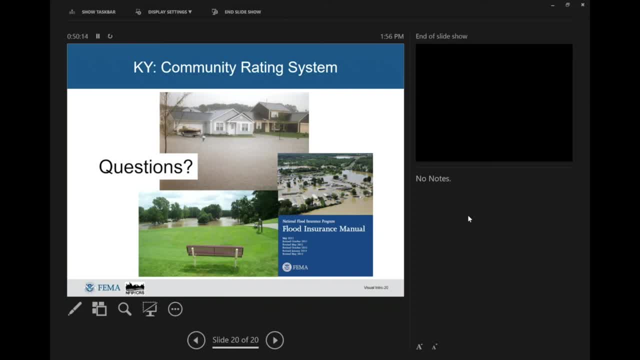 everybody else together. i like to say that the best crs coordinators are those that are great with logistics. they can farm out things and then bring it back together, so it can be anybody that they appoint. it could be your emergency manager. i have building inspectors. i have um in augusta. 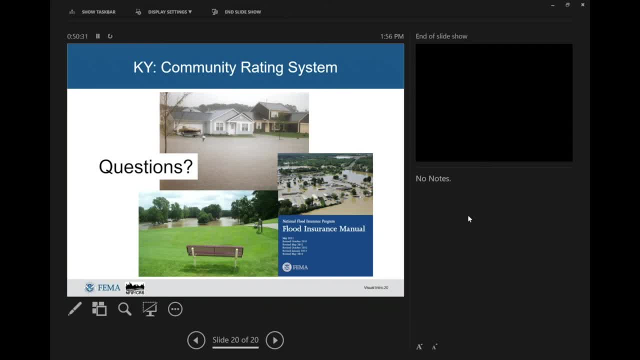 it's who's like the clerk right. is that her title? the city clerk in augusta, gretchen, i believe? so, yeah, yeah. so i mean we, we have communities that have really limited staff, so that they have people that do more than one thing and they add that and obviously those folks. 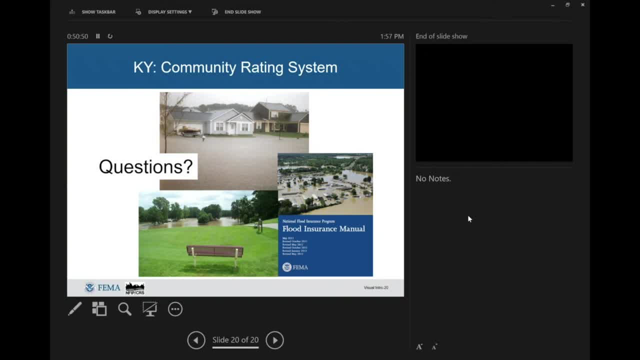 that maybe they're not the floodplain manager. we will do everything we can to help them be effective and successful as a crs coordinator, but it can be anybody that the community deems they. we just ask them to name one person, because i don't. it's not as effective if i have to contact five to seven. 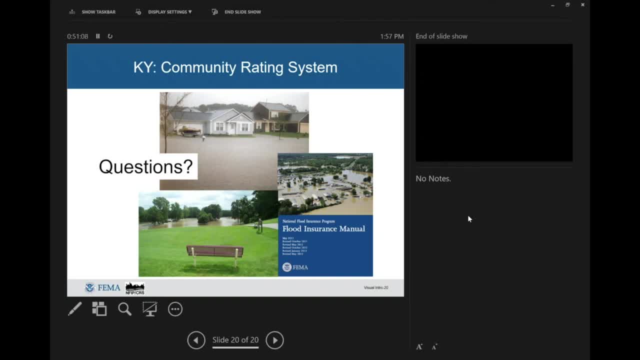 people in the community to get documentation, as if, um, the community has one person for all the documentation to come to and then they they communicate with me. perfect thanks, christina. um, it doesn't look like we had any other questions come in, so i'm going to switch back over and 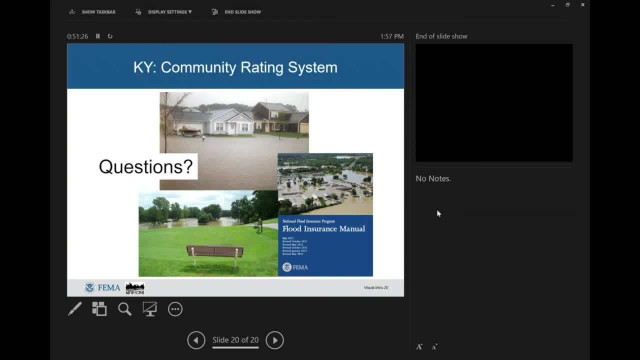 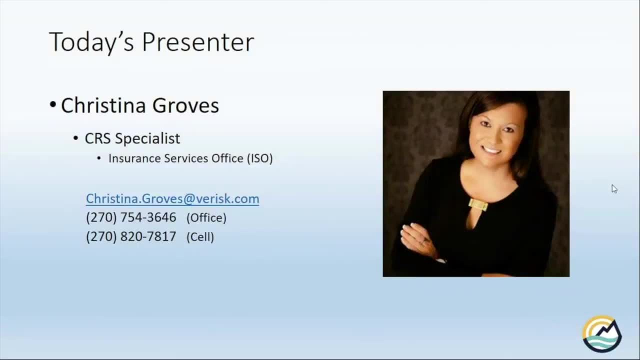 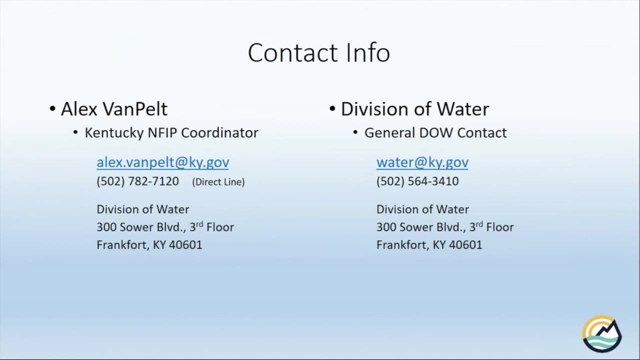 start showing my screen again. thank you. thank you so much. you can just sit back and relax for a minute, so all right, thanks, alex. okay, um, the last thing, guys. i only have two more slides before we wrap up. um, so i wanted to share my contact info with everybody again. um, if you have problems, if you have questions with anything that. 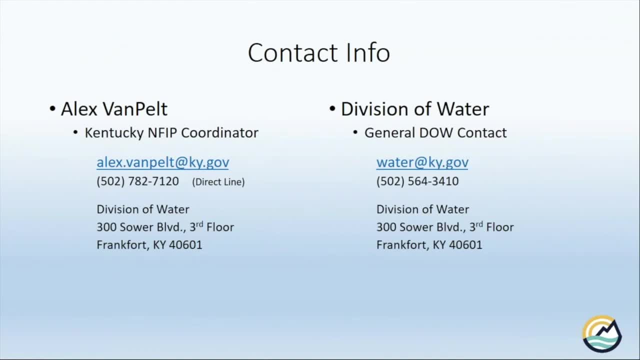 was shared today. so if you want to reach out to dr christina again, if you want to talk to me about scheduling a calf to start, you know the entry process um into joining or participating into crs. if you just want to talk more about what activities are credible or things like that, you can reach me. 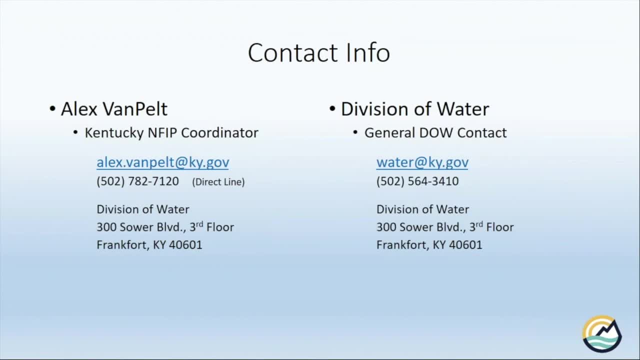 um, best way to do it is email. i'm in the field quite often, so emailing me at that kygov is the best way to get me. i've also listed my direct line. if you leave me a message, i will call you back at some point. i can't guarantee when that's going to be. the other way to get a hold of me, though, is also you can. 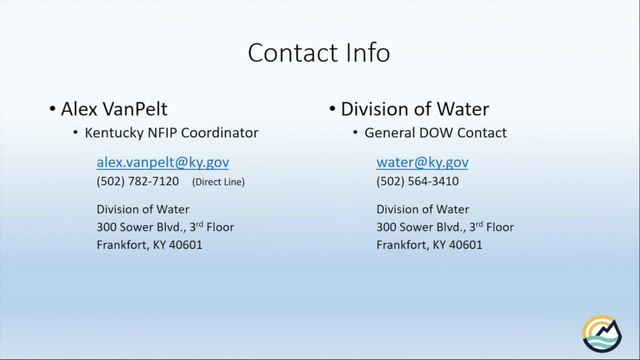 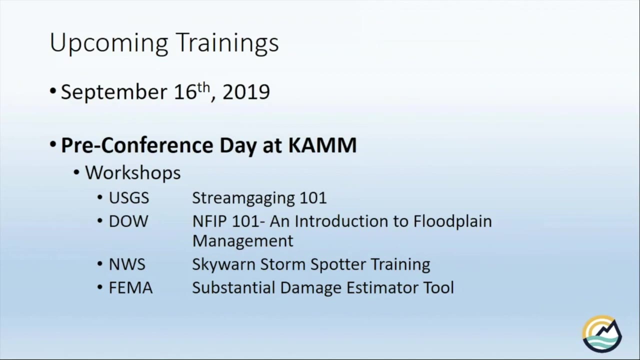 reach out to the, just the general contact line at division water, so water at KY gov, or the general phone number. if you call that and ask for me or ask to the floodplain coordinator, they're going to put you in touch with me. and the last thing I want to share with you guys, so if you're looking for more training next, 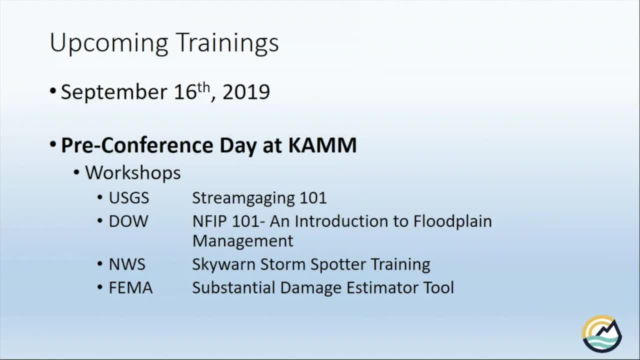 week is a really great opportunity. so next week- Christina mentioned cam, which is the Kentucky Association of mitigation managers. our conference is next week, on the 17th through the 19th, but they're also doing what they call a pre-conference day. so Monday, the 16th, they are doing several workshops. 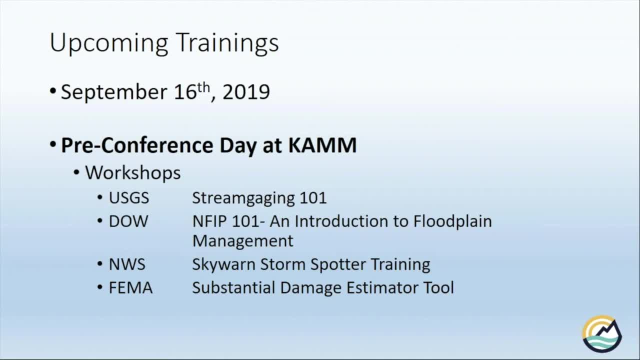 throughout the day that are going to be covering several different topics and I just wanted to call your all the attention to them. USGS, which is the US Geological Survey. they're doing a stream gauging workshop. a 101: I'm offering a NFIP 101 introduction to floodplain management. 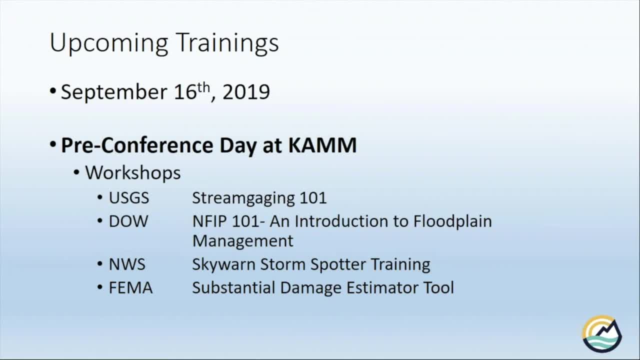 in the morning National Weather Service is doing a Skywarn, which is a storm spotter training, and then FEMA- one of the folks from FEMA region 4 in Atlanta is actually doing a demonstration of the substantial damage estimator tool, which is really useful for local officials whenever it comes to doing substantial 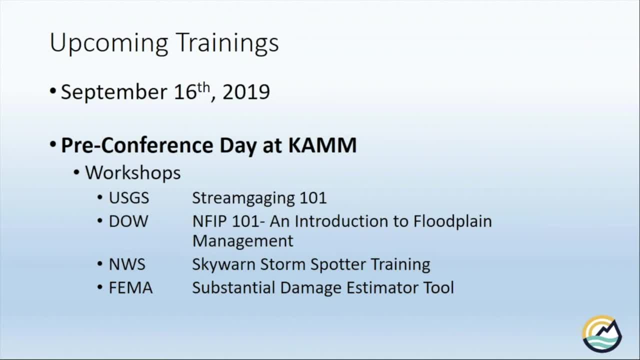 damage determinations after a flood or something like that. so several really great trainings and workshops that are going to be happening throughout the week. so that's why I'm here today, because I just wanted to share that with you and to give you all a sense of what we're working on, and it's important that. 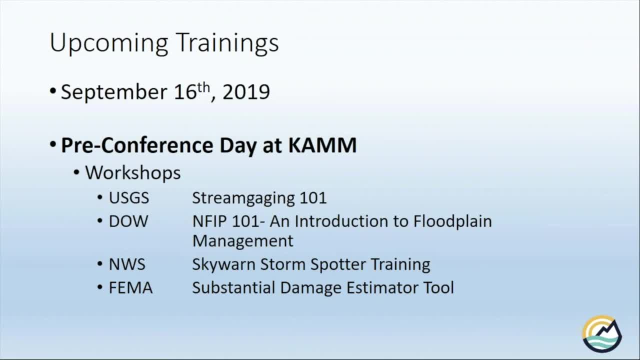 you get a chance to get a chance to take part in these workshops. anybody who wants to can attend those. they are absolutely free. you don't have to even attend the whole conference or become a member of cam to do those. so if you guys know of anybody who would be interested in one of those, please share it with them. we. 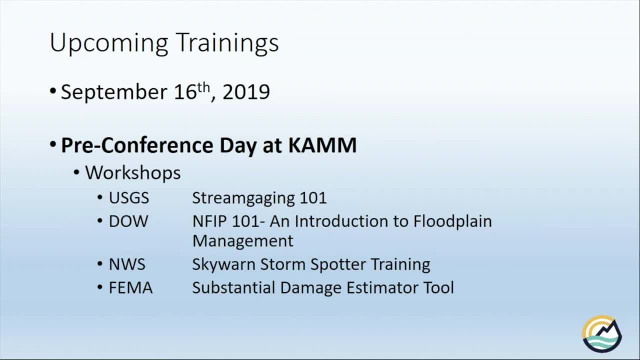 would love to have them and with that guys. that is everything we have today. I'm going to stick around for another couple minutes to take questions, so I'm going to sit here and keep watching the chat box, but, if nothing else, guys coming and spending about an hour in time with us. so thank you very much. everybody, have a good day. you. 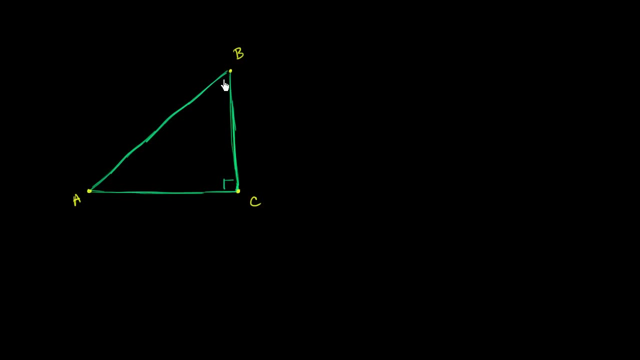 We see, in a triangle- or I guess we know, in a triangle there's three angles, And if we're talking about a right triangle, like the one that I've drawn here, one of them is going to be a right angle, And so we have two other angles to deal with. 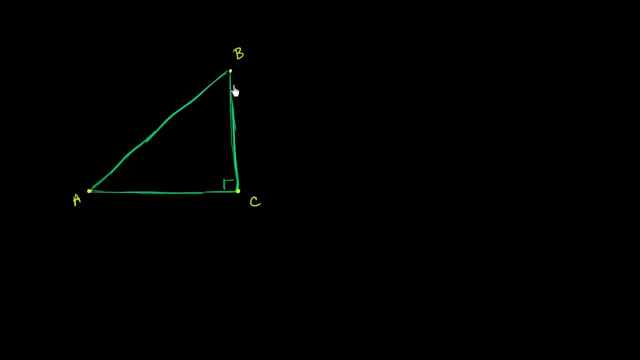 And what I want to explore in this video is the relationship between the sine of one of these angles and the cosine of the other, the cosine of one of these angles and the sine of the other. So to do that, let's just say that this angle